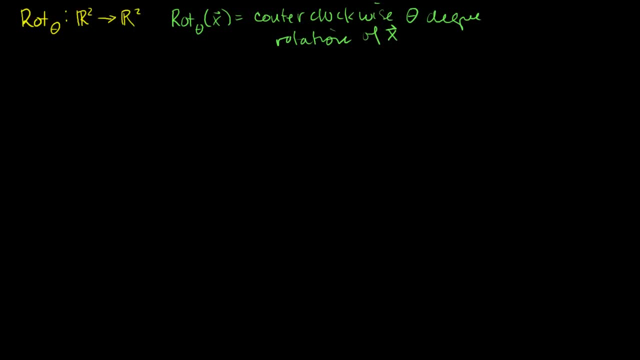 need to make sure there's an actual linear transformation. I'll just do that visually because I actually don't even have a math map. OK, I don't have a mathematical definition for this yet. This is about as good as I've given you. 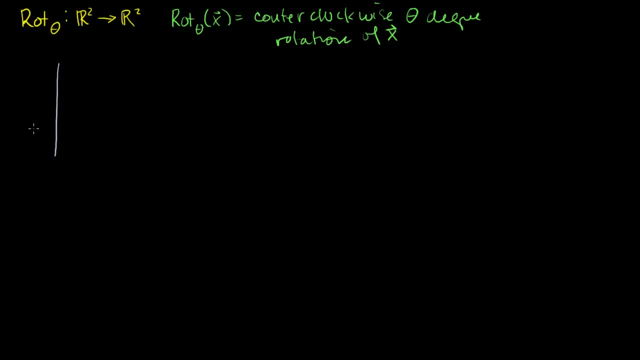 So let me just draw some really fast axes right here. I have to draw them a little bit neater than that. That's my vertical axes. That's my horizontal axes. I could call this, I'll call this one the x1 and I'll call. 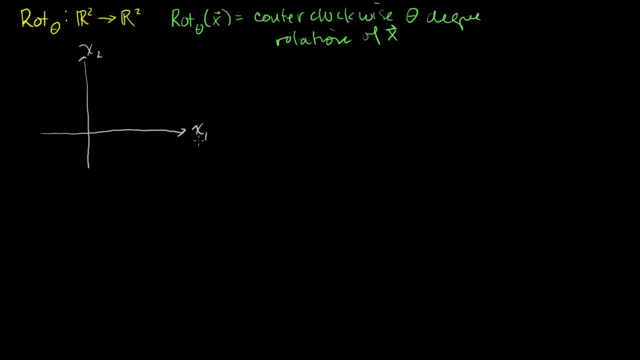 this the x2 axis. In the last video I called them the x and the y, but you know, this is the first component of our vectors. This is our second component of our vectors, And so if I have some vector x like that, 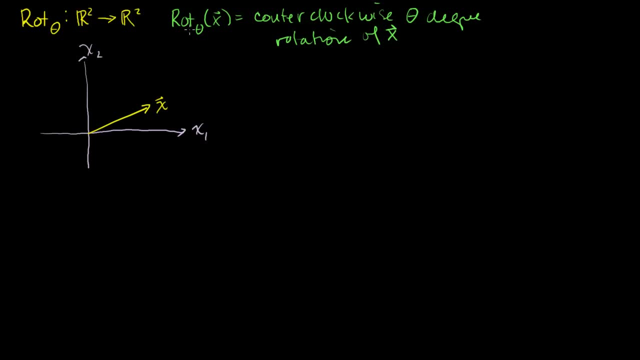 We know that a rotation of this, a counterclockwise rotation of this, will look like this. I'll do the rotations in blue. It will look like this: Where this angle right here is theta. So this right here is the rotation for an angle of theta. 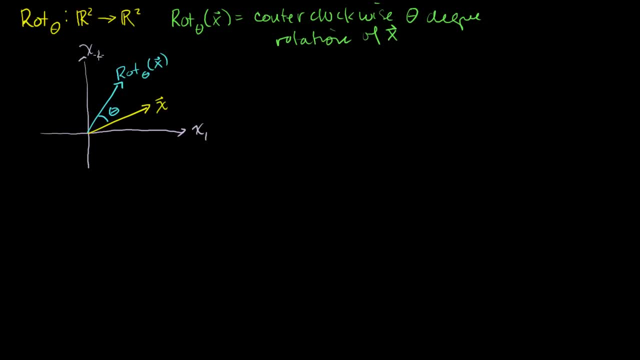 of x. That's what this vector right here is. So what do we have to do to make sure that this is a linear combination? We have to show two things. We have to show that the transformation, so the rotation through x, Through theta, of the sum of two vectors 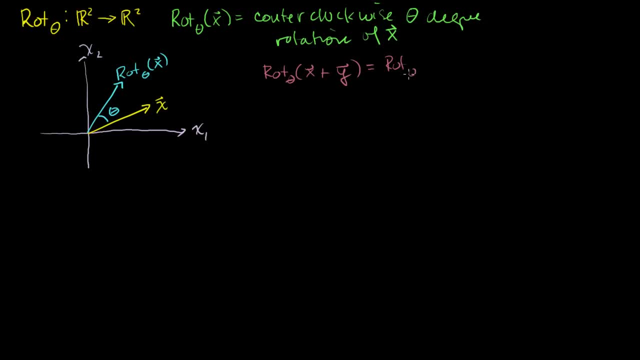 It's equivalent to the sum of each of their individual rotations, The rotation of the vector x plus the rotation of the vector y, And I'll just show that to you visually. This is the vector x. Let's say that the vector y looks something like. let me 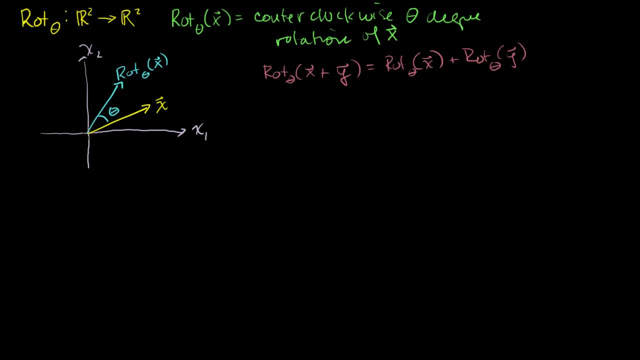 draw. well, I'll draw both of the original vectors in yellow. So let's say, the vector y looks like that, So that's y. So what's x plus y? So let's put heads to tails If we just shift y up here. 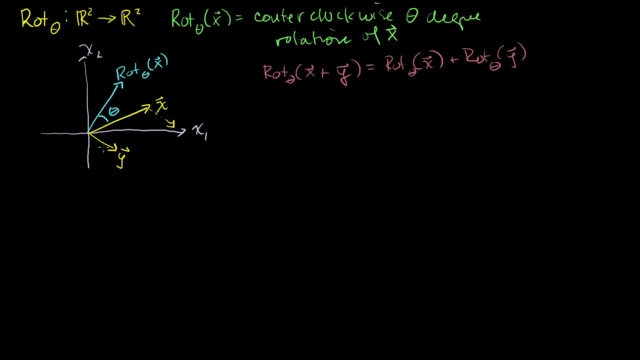 If you just shift y up there, that's also vector y, Not drawn in standard position, But x plus y would then well, it would look pretty close to this. I'm not drawing it, Let me draw it a little bit neater. 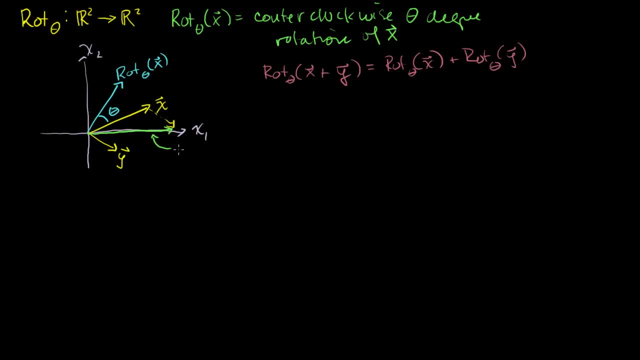 x plus y would look like that. That would be the vector x plus y. And what would its rotation look like through an angle of theta? Well, its rotation if you just rotate this guy through an angle of theta, I'm just approximating. 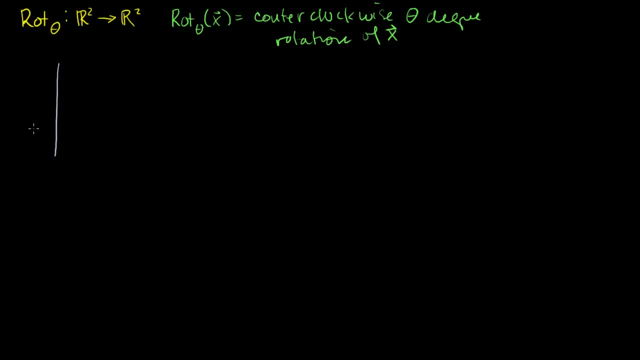 So let me just draw some really fast axes right here. I have to draw them a little bit neater than that. That's my vertical axes. That's my horizontal axes. I could call this, I'll call this one the x1 and I'll call. 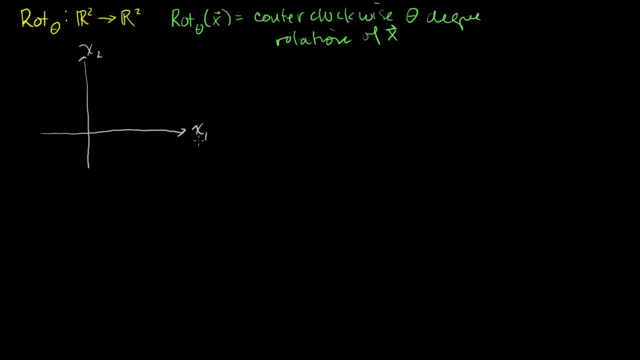 this the x2 axis. In the last video I called them the x and the y, but you know, this is the first component of our vectors. This is our second component of our vectors, And so if I have some vector x like that, 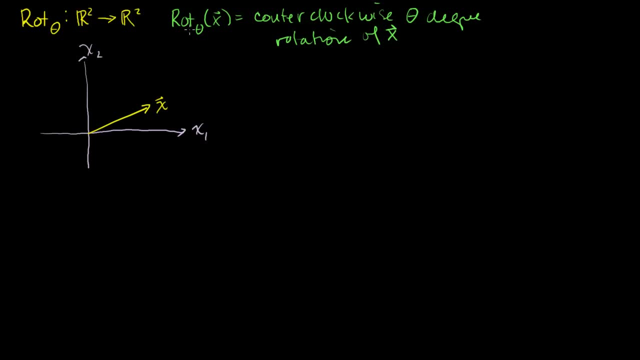 We know that a rotation of this, a counterclockwise rotation of this, will look like this. I'll do the rotations in blue. It will look like this: Where this angle right here is theta. So this right here is the rotation for an angle of theta. 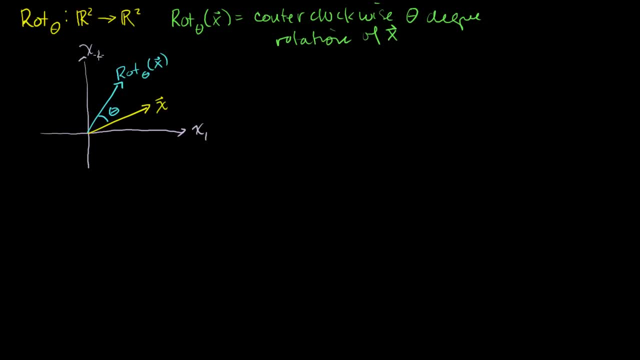 of x. That's what this vector right here is. So what do we have to do to make sure that this is a linear combination? We have to show two things. We have to show that the transformation, so the rotation through x, Through theta, of the sum of two vectors 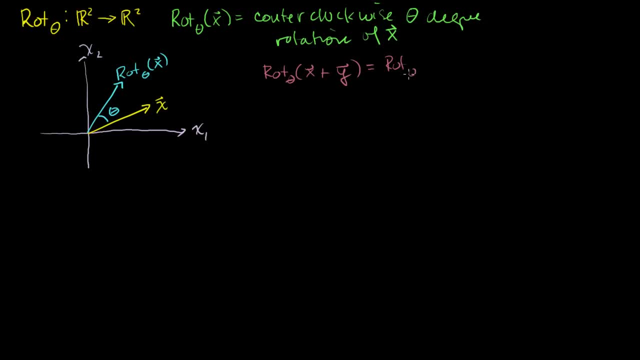 It's equivalent to the sum of each of their individual rotations, The rotation of the vector x plus the rotation of the vector y, And I'll just show that to you visually. This is the vector x. Let's say that the vector y looks something like. let me 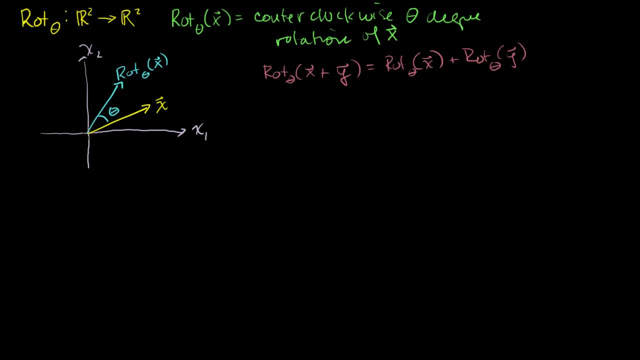 draw. well, I'll draw both of the original vectors in yellow. So let's say, the vector y looks like that, So that's y. So what's x plus y? So let's put heads to tails If we just shift y up here. 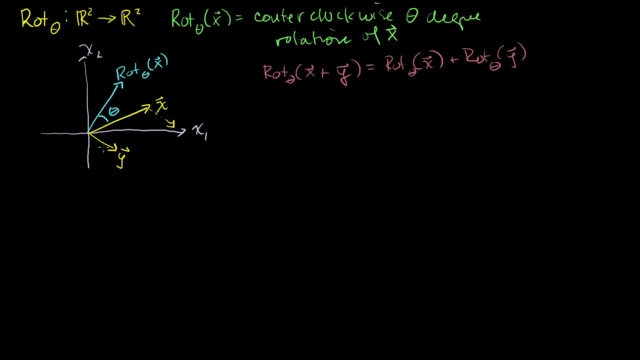 If you just shift y up there, that's also vector y, Not drawn in standard position, But x plus y would then well, it would look pretty close to this. I'm not drawing it, Let me draw it a little bit neater. 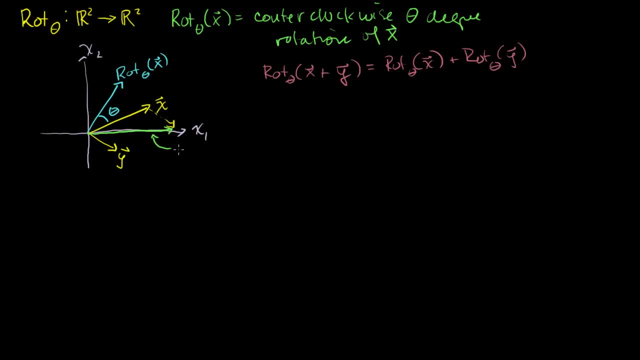 x plus y would look like that. That would be the vector x plus y. And what would its rotation look like through an angle of theta? Well, its rotation if you just rotate this guy through an angle of theta, I'm just approximating. 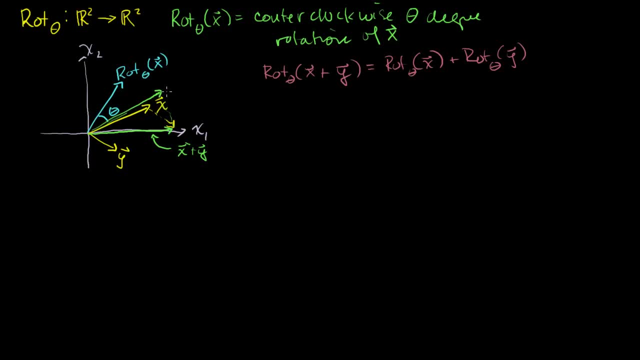 It would look something like this, It would look something like that. So this right here, this would be the rotation through an angle of theta of x plus y. Now let's see if that's the same thing as if we rotate x and rotate y and then add them together. 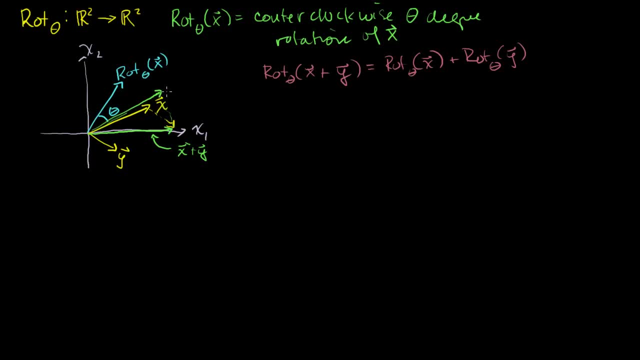 It would look something like this, It would look something like that. So this right here, this would be the rotation through an angle of theta of x plus y. Now let's see if that's the same thing as if we rotate x and rotate y and then add them together. 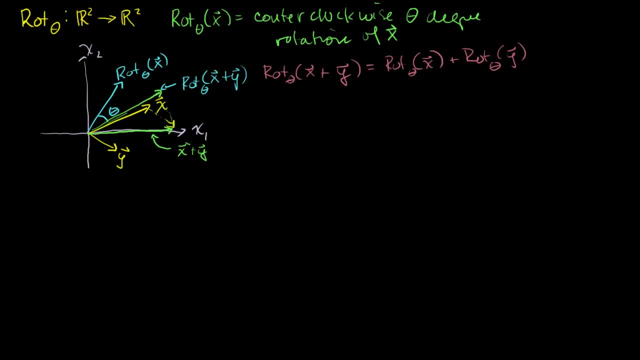 So what's y if we rotate it through an angle of theta? If we rotate y through an angle of theta, it's going to look something like It's all approximation. I should be doing it with a ruler and a protractor. Maybe it looks something like this. 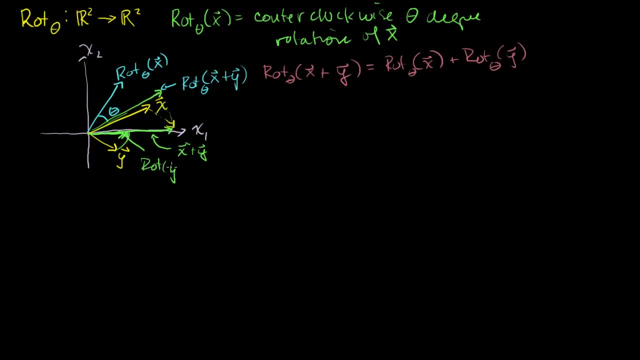 So this is right here. That's the rotation of y through an angle of theta. That's the same theta that I've been doing the whole time. Let me make it in a color that you can actually see. So that's that vector, right there. 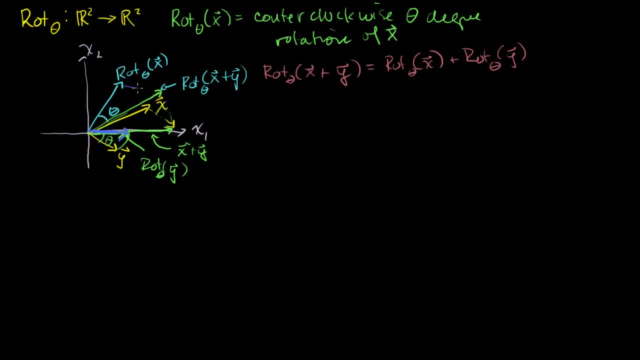 The rotation of x was right there. So if we add the rotation of x plus the rotation of y- I'm kind of fudging it a little bit, but I think you get the idea You actually get. So this is the rotation of x. 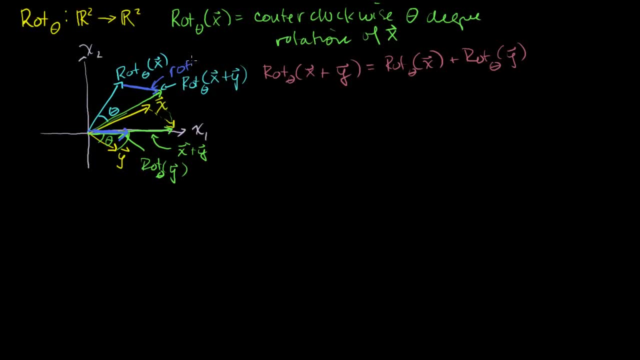 This is the rotation of x plus the rotation of y, Rotation of our vector y, You actually get the rotation of x plus y. So at least visually, it satisfied that first condition. Now the second condition that we need for this to be a 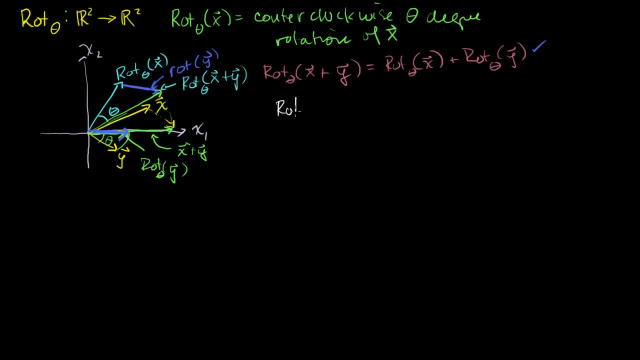 valid linear transformation is that the rotation through an angle of theta of a scaled up version of a vector. it should be equal to a scaled up version of the rotated vector And I'll just do another visual example here. So let's say this is my vertical axis. 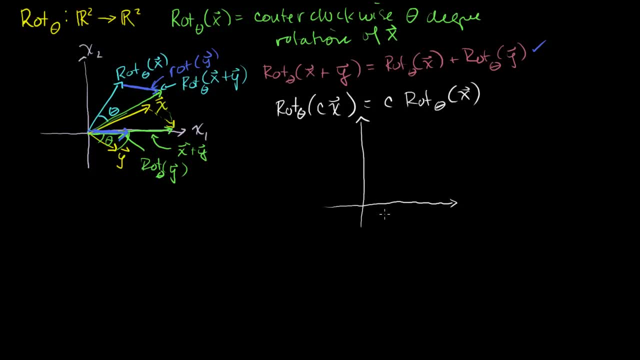 That's my horizontal axis, And let me say that this is my vector x. Now let's draw a scaled up version of it. So a scaled up version of x. Maybe it's just like x, but it gets scaled up a little bit. 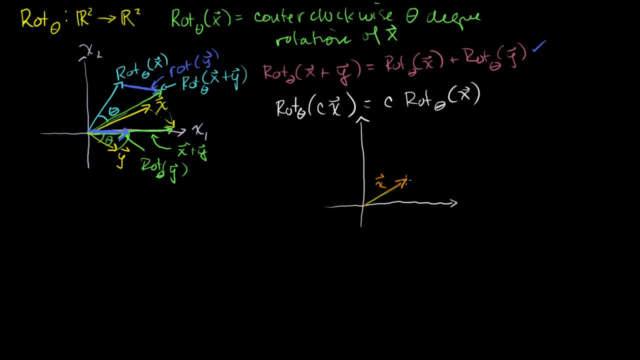 So it goes all the way out here. So this is my c times x, And now we're going to rotate that through an angle of theta. So if we rotate that through an angle of theta, you'll get a vector that looks something like this: 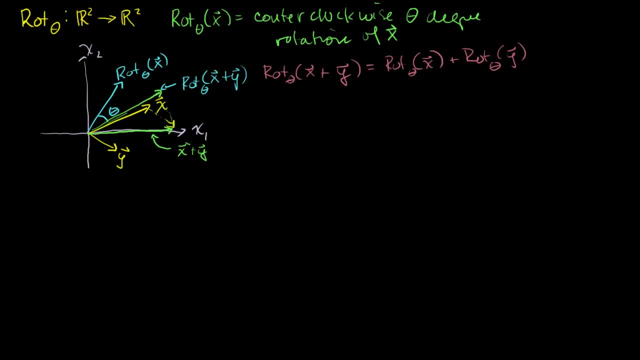 So what's y if we rotate it through an angle of theta? If we rotate y through an angle of theta, it's going to look something like It's all approximation. I should be doing it with a ruler and a protractor. Maybe it looks something like this. 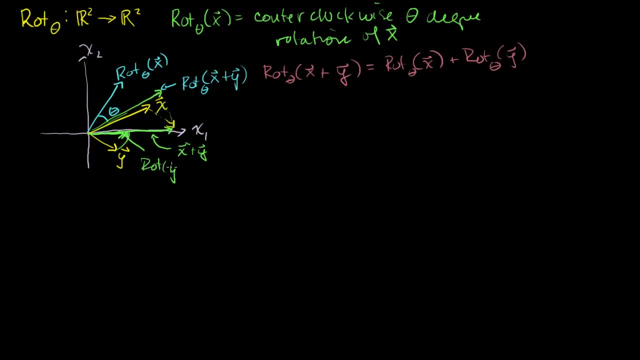 So this is right here. That's the rotation of y through an angle of theta. That's the same theta that I've been doing the whole time. Let me make it in a color that you can actually see. So that's that vector, right there. 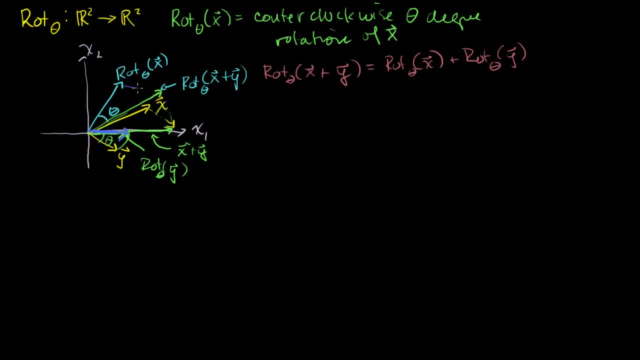 The rotation of x was right there. So if we add the rotation of x plus the rotation of y- I'm kind of fudging it a little bit, but I think you get the idea You actually get. So this is the rotation of x. 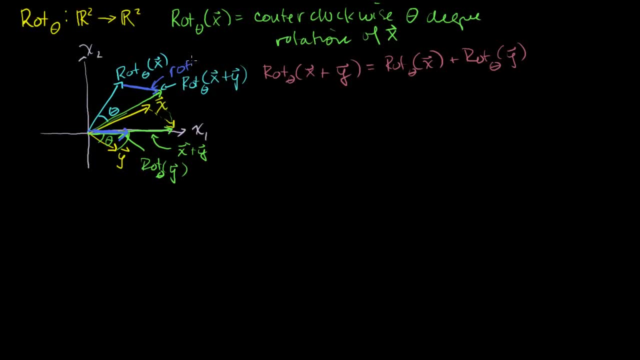 This is the rotation of x plus the rotation of y, Rotation of our vector y, You actually get the rotation of x plus y. So at least visually, it satisfied that first condition. Now the second condition that we need for this to be a 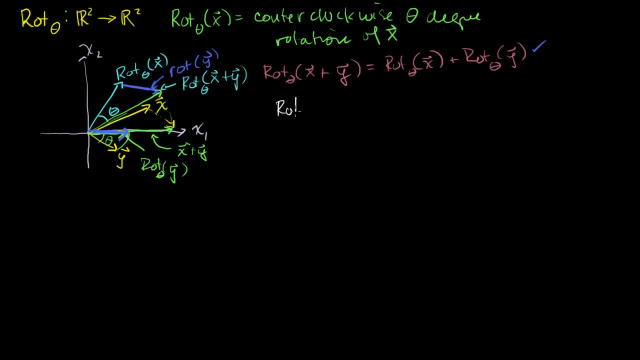 valid linear transformation is that the rotation through an angle of theta of a scaled up version of a vector. it should be equal to a scaled up version of the rotated vector And I'll just do another visual example here. So let's say this is my vertical axis. 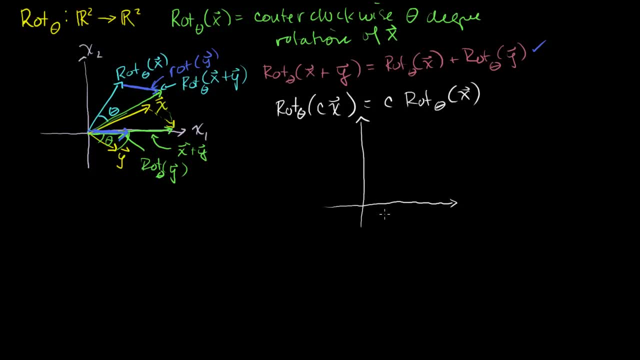 That's my horizontal axis, And let me say that this is my vector x. Now let's draw a scaled up version of it. So a scaled up version of x. Maybe it's just like x, but it gets scaled up a little bit. 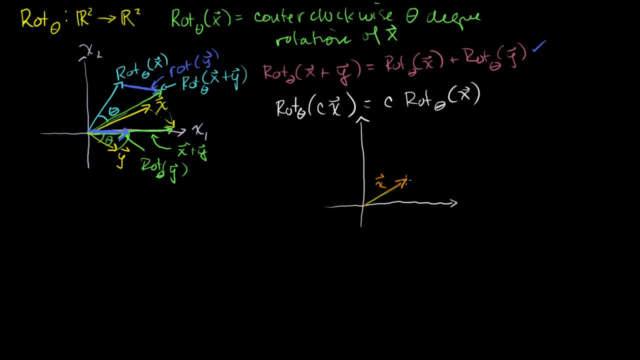 So it goes all the way out here. So this is my c times x, And now we're going to rotate that through an angle of theta. So if we rotate that through an angle of theta, you'll get a vector that looks something like this: 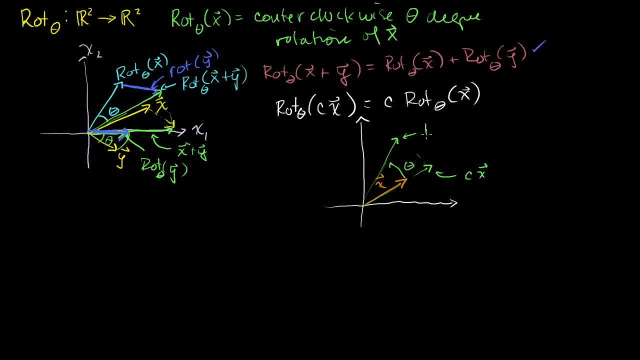 Rotating it counterclockwise. So this vector right here is the rotation by an angle of theta, counterclockwise of cx. That's what this is right there. Now, what happens if we take the rotation of x first? So if we just rotate x first, we're going to get this. 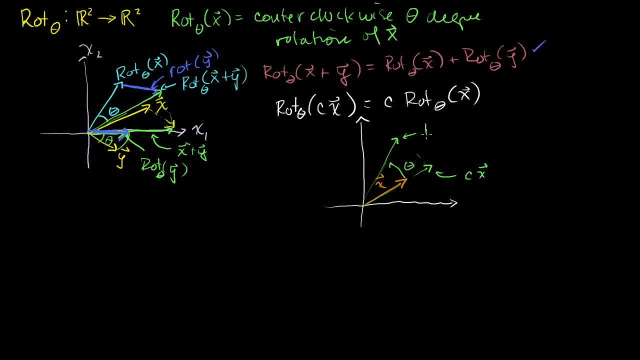 Rotating it counterclockwise. So this vector right here is the rotation by an angle of theta, counterclockwise of cx. That's what this is right there. Now, what happens if we take the rotation of x first? So if we just rotate x first, we're going to get this. 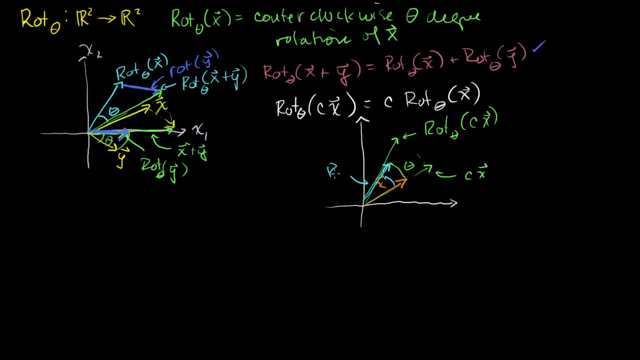 vector right here. So this right here is just the rotation through an angle of theta of x, And then we scale it up. Well, we see, it's the same thing. If this scaled up to that, when you multiply it by c, then this thing is going to scale up to that. when 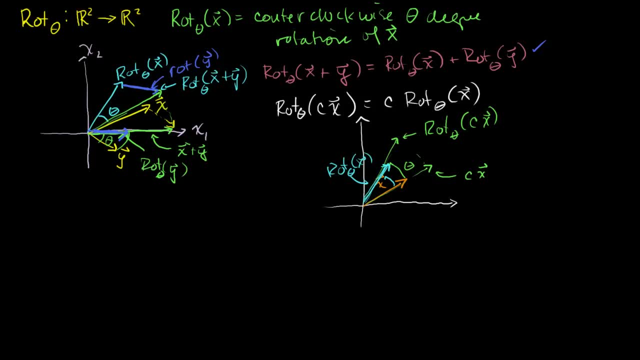 you multiply it by c. So at least visually, I've shown you that this is satisfied. So rotation definitely is a linear transformation, at least the way I've shown you. Now let's actually construct a mathematical definition for it. Let's actually construct a matrix that will perform an. 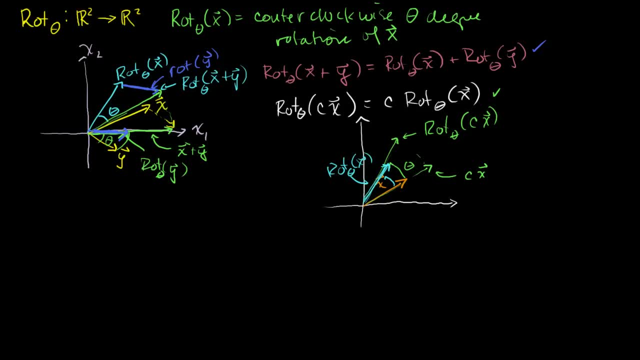 polynomial in px form the transformation. So I'm saying that my rotation transformation from R2 to R2 of some vector x can be defined as some 2 by 2 matrix. And it's 2 by 2 because it's a mapping from R2 to R2, times. 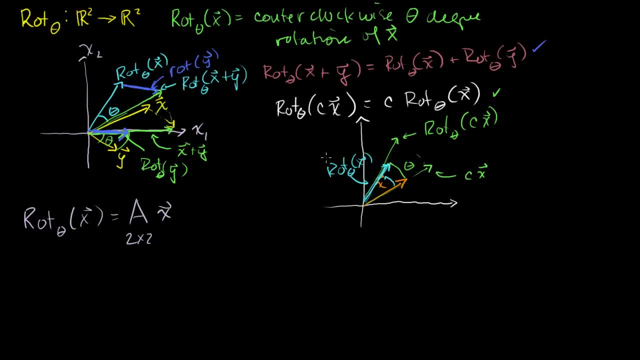 any vector x, And I'm saying I can do this because I've at least shown you visually that it is indeed a linear transformation. And how do I find A? Well, I start with- since this was mapping from R2, I start. 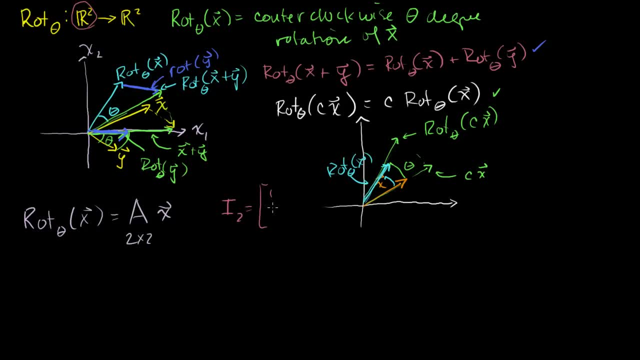 with the identity matrix in R2, which is 1,, 0,, 0,, 1.. Its columns are the basis vectors for R2.. We refer this one as E1 and this column vector as E2.. And to figure out A, we essentially just perform the 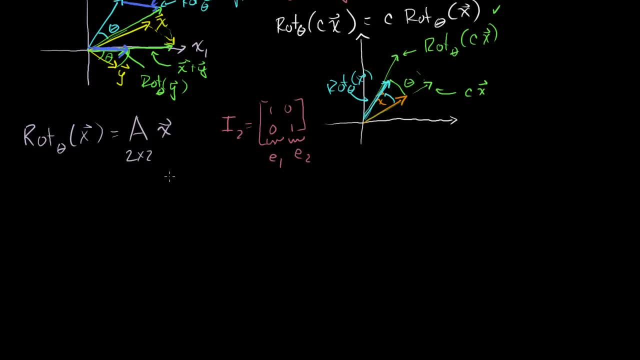 transformation on each of these columns. So let me write that. So A, Our matrix. A is going to be the first column of it is going to be our rotation transformation performed on the vector 1, 0.. And our second column is going to be the rotation. 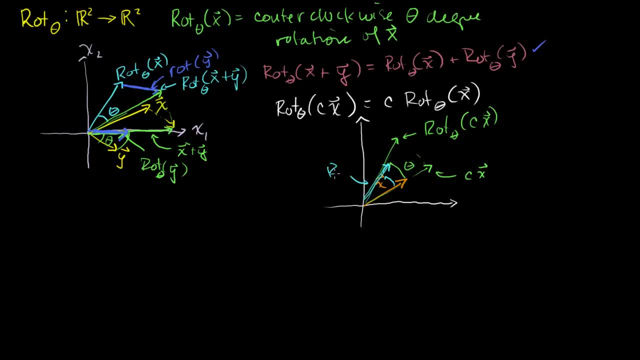 vector right here. So this right here is just the rotation through an angle of theta of x, And then we scale it up. Well, we see, it's the same thing. If this scaled up to that, when you multiply it by c, then 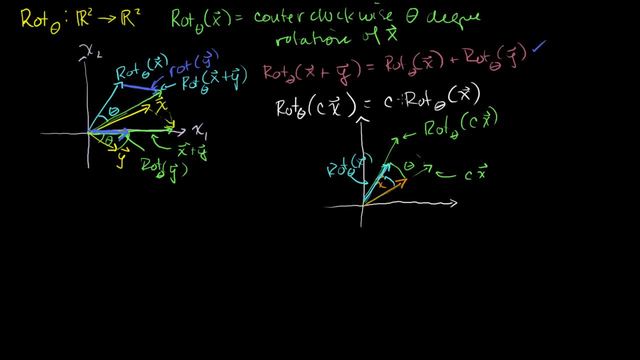 this thing is going to scale up to that when you multiply it by c. So at least visually, I've shown you that this is satisfied. So rotation definitely is a linear transformation, at least the way I've shown you. Now let's actually construct a mathematical. 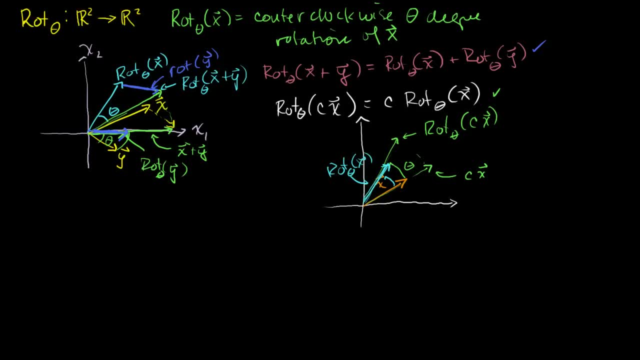 definition for it. Let's actually construct a matrix that will perform a linear transformation, form the transformation. So I'm saying that my rotation transformation from R2 to R2 of some vector x can be defined as some 2 by 2 matrix. 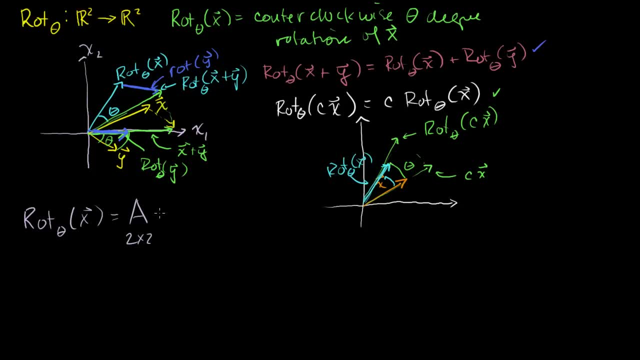 And it's 2 by 2, because it's a mapping from R2 to R2, times any vector x. And I'm saying I can do this because I've at least shown you visually that it is indeed a linear transformation. And how do I find A? 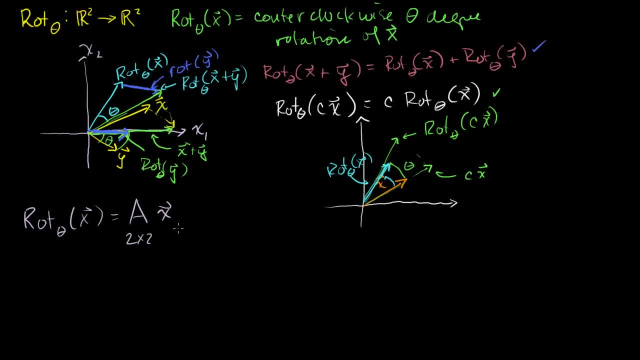 Well, I start with, since this was mapping from R2, I start with the identity matrix in R2, which is 1, 0, 0, 1.. Its columns are the basis vectors for R2.. We refer this one as E1 and this column vector as E2.. 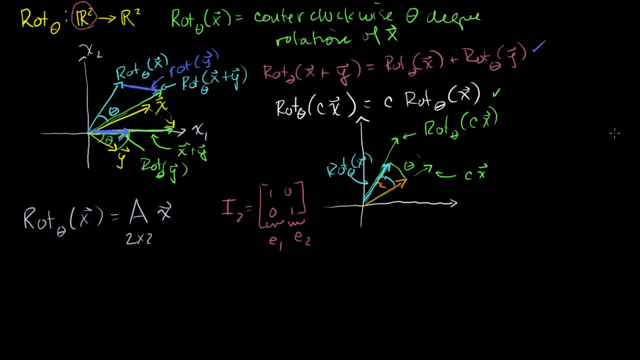 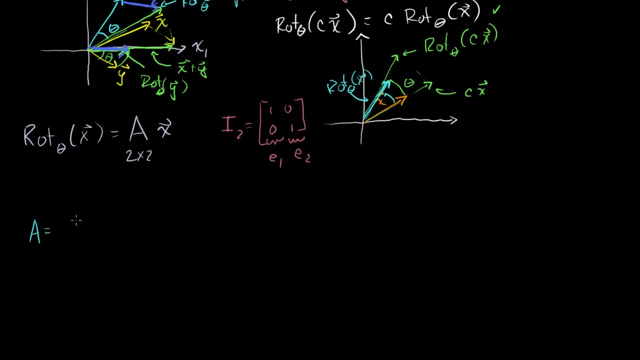 And to figure out A, we essentially just perform the transformation on each of these columns. So let me write that. So A, Our matrix. A is going to be the first column of. it is going to be our rotation transformation, performed on the vector 1, 0. 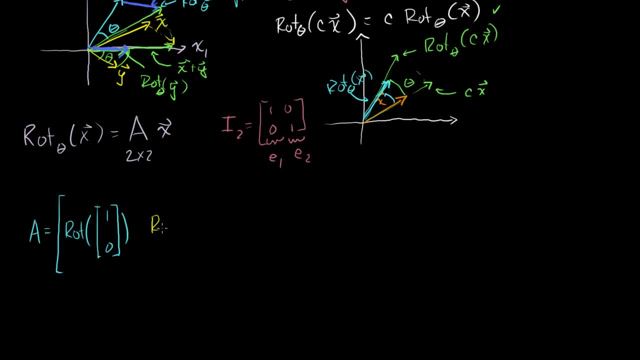 And our second column is going to be the rotation transformation. there's a little theta here that I'm forgetting to write times, the second column, vector times, or the transformation of that one: 0, 1.. This is what our A is going to look like. 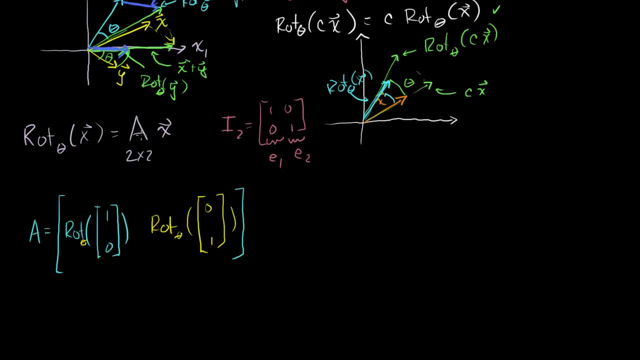 So how do we figure out what these are? I'm trying to get to some numbers and this doesn't get me there, so let's try to do that. Let me draw some more axes here. Let me pick a different color. I'll do it in gray. 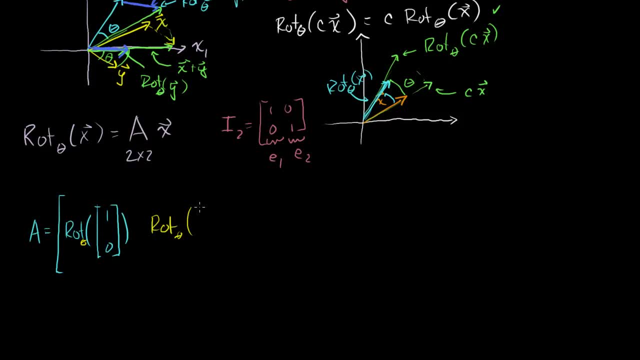 transformation. there's a little theta here that I'm forgetting to write: times, the second column, vector, times, or the transformation of that one: 0, 1.. This is what our A is going to look like, So how do we figure out what these are? 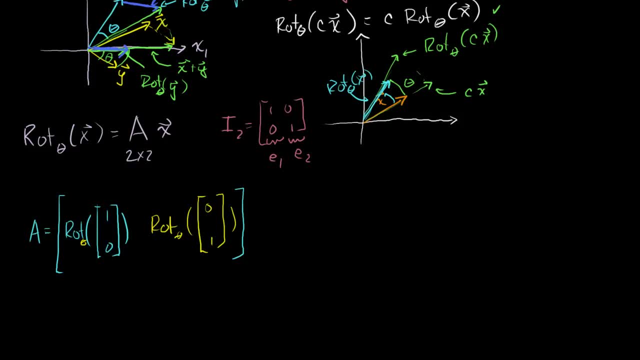 I'm trying to get to some numbers and this doesn't get me there. so let's try to do that. Let me draw some more axes here. Let me pick a different color. I'll do it in gray. So that is my vertical axes, that is my horizontal axes, and 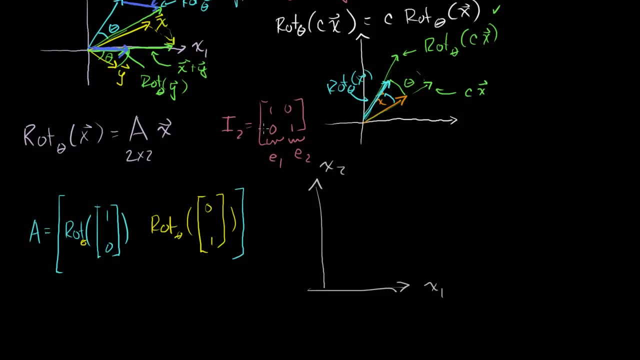 I could call this the x1 axis and this is the x2 axis. Now, this basis vector E1, what does it look like? Well, it's 1 in the horizontal axis, Horizontal x1 is 1 and x2 is 0.. 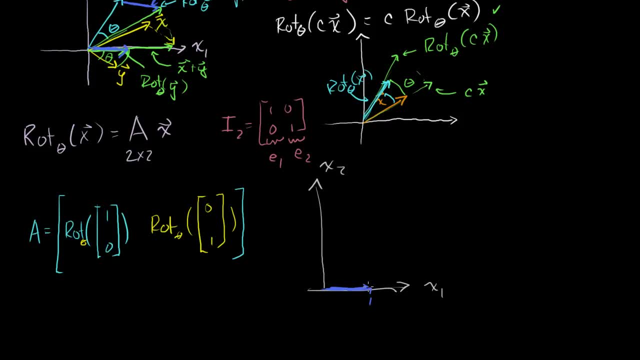 So if this is 1 out here, E1 will look like that. Let me do it in a more vibrant color. E1 will look like that. right there Now, if I'm rotating, let me write what E2 looks like. 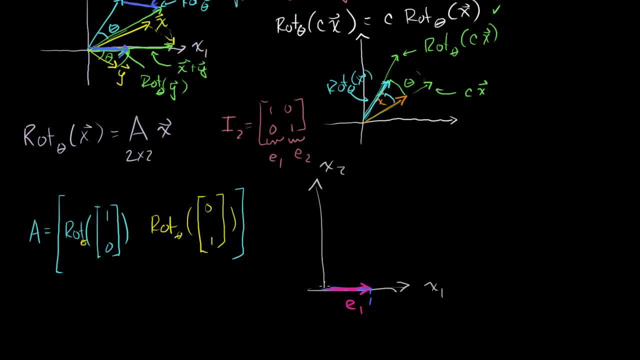 E2 would look like. I'll do it in yellow: E2 would look like this, right here: E2.. That's that vector 0, 1.. This is 1 in our vector. This is in our x2 direction. 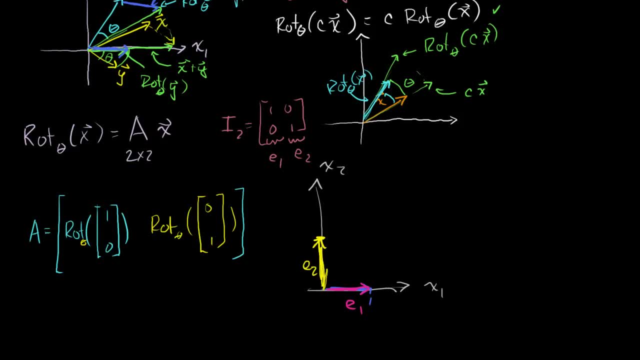 Now, if I rotate E1 by an angle theta, what will it look like? So if I rotate E1 an angle of theta, I'll do it in this color right here. it will still have a length of 1,, but it'll be. 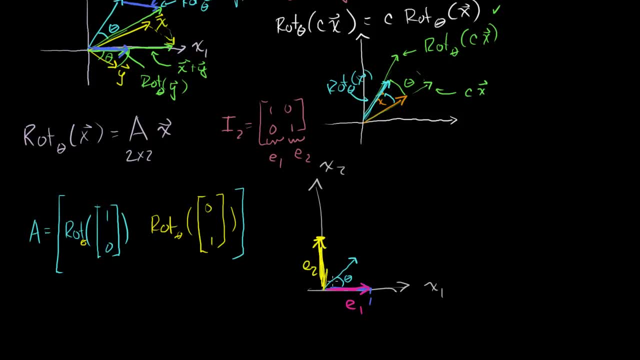 rotated like that And that angle right there is theta. So this right here is the rotation of E1 by theta. These are all vectors, of course. That's what that is. Now, what are the coordinates for this, or how do we specify? 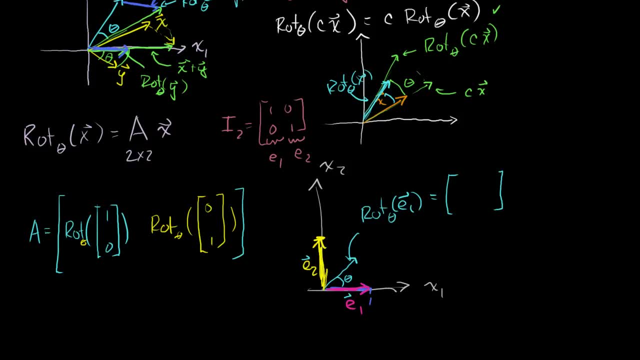 this new vector. Well, we can break out a little bit of our trigonometry. It's new x1 coordinate. we could call it or. its x1 entry is going to be this length right here. It's going to be this length, right here. 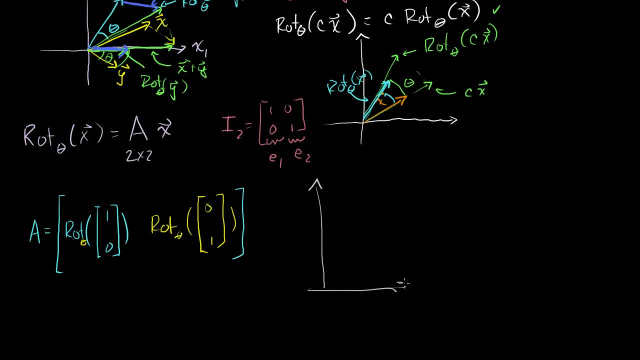 So that is my vertical axes, that is my horizontal axes, and I could call this the x1 axis and this is the x2 axis. Now, this basis, vector E1, what does it look like? Well, it's 1 in the horizontal axis. 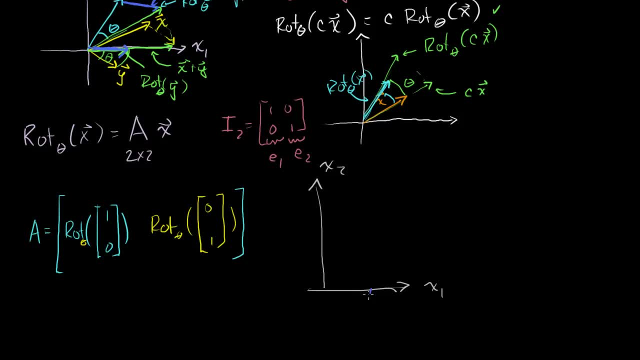 Horizontal x1 is 1 and x2 is 0. So if this is 1 out here, E1 will look like that. Let me do it in a more vibrant color. E1 will look like that. right there Now, if I'm rotating, let me write what E2 looks like. 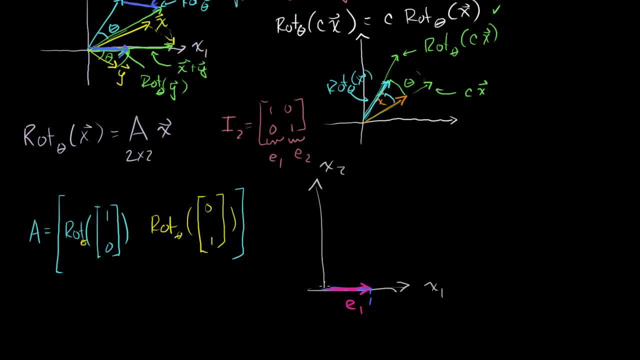 E2 would look like. I'll do it in yellow: E2 would look like this, right here: E2.. That's that vector 0, 1.. This is 1 in our vector. This is in our x2 direction. 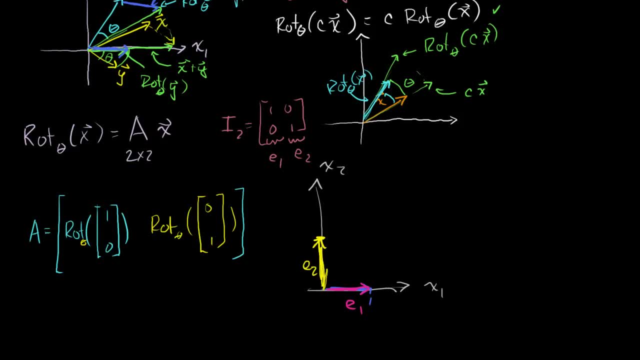 Now, if I rotate E1 by an angle theta, what will it look like? So if I rotate E1 an angle of theta, I'll do it in this color right here. it will still have a length of 1,, but it'll be. 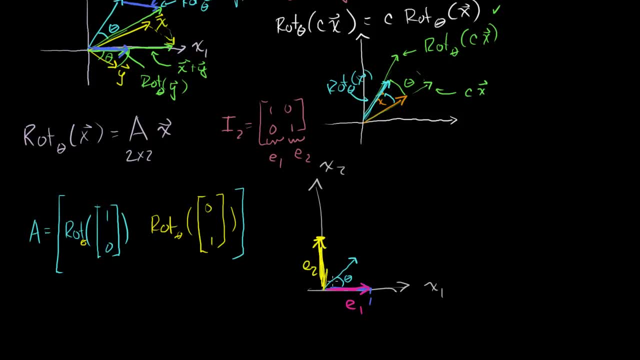 rotated like that And that angle right there is theta. So this right here is the rotation of E1 by theta. These are all vectors, of course. That's what that is. Now, what are the coordinates for this, or how do we specify? 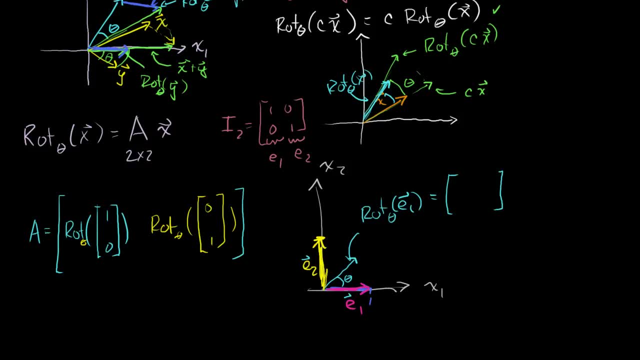 this new vector. Well, we can break out a little bit of our trigonometry. Its new x1 coordinate, we could call it or its x1 entry is going to be this length, right here. So if we draw a right triangle, it is the side that is. 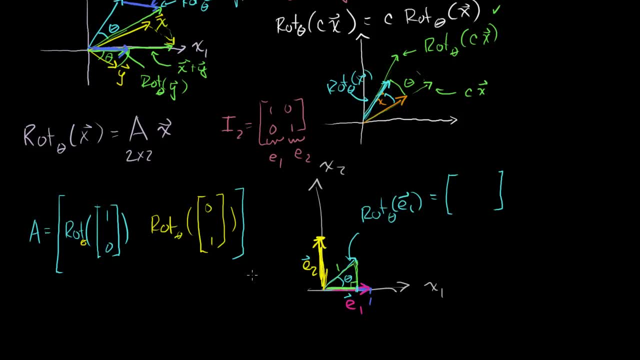 adjacent to theta. This side is the hypotenuse, which is length 1.. So how do we figure out this side? If we call this side the adjacent side, then we'll be able to find the adjacent side. The adjacent side over the hypotenuse, adjacent over the. 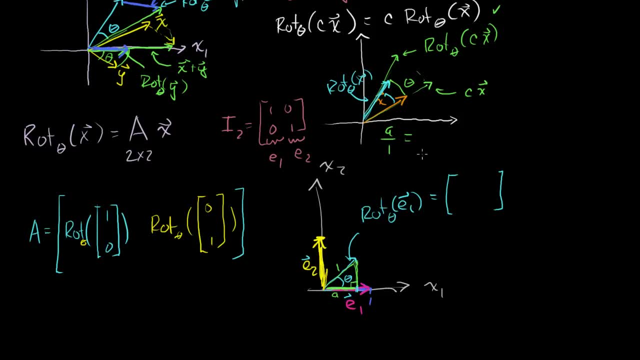 hypotenuse, which is just 1, is equal to the cosine of theta That comes from SOH CAH TOA. Let me write that Cosine is adjacent over hypotenuse And the adjacent side is going to be our new x1 coordinate. 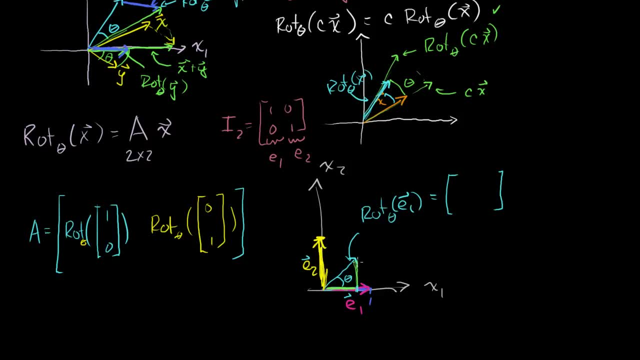 So if we draw a right triangle, it is the side that is adjacent to theta. This side is the hypotenuse, which is length one. So how do we figure out this side? If we call this side the adjacent side, side over the hypotenuse, which is just 1, is equal to. 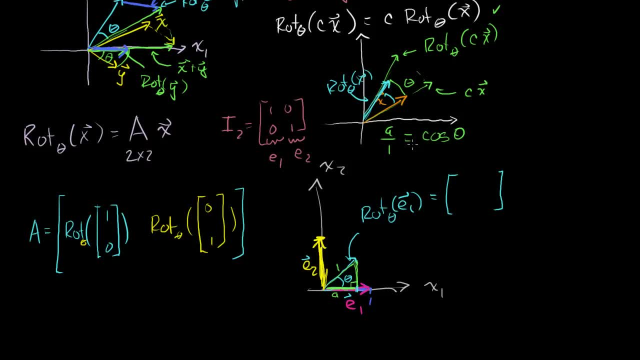 the cosine of theta That comes from SOH CAH TOA. Let me write that Cosine is adjacent over hypotenuse And the adjacent side is going to be our new x1 coordinate. Well, we can obviously ignore that 1.. 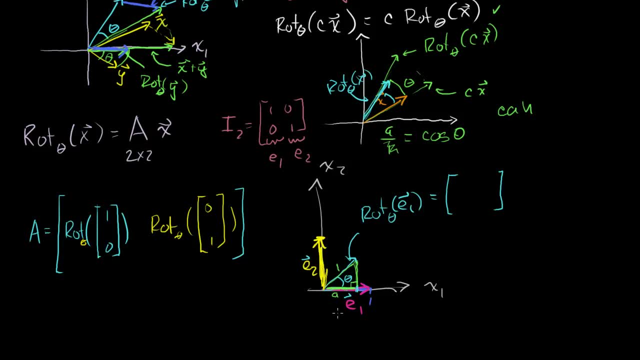 a divided by 1 is equal to cosine theta, which means that a is equal to cosine theta, which means that this length of our rotated vector is equal to cosine theta. Its horizontal component or its horizontal coordinate is equal to cosine of theta. Now, if we take what's its vertical component going to be? 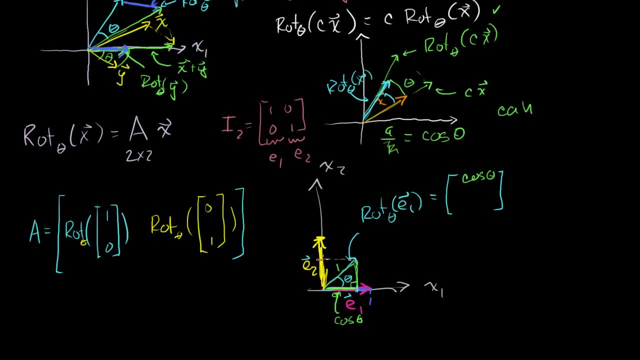 it's going to be this height right here. It's going to be that height right there, which is the same thing as that height. It's going to be that height right there. Or we could say sine of theta. Let me call this the opposite. 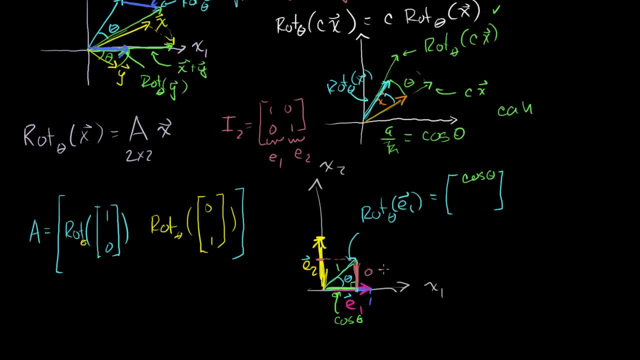 Sine of theta is equal to the opposite over 1.. So this is going to be equal to sine of theta. This over 1, which is just this, is equal to sine of theta from SOH CAH TOA. So this vertical component is equal to sine of theta. 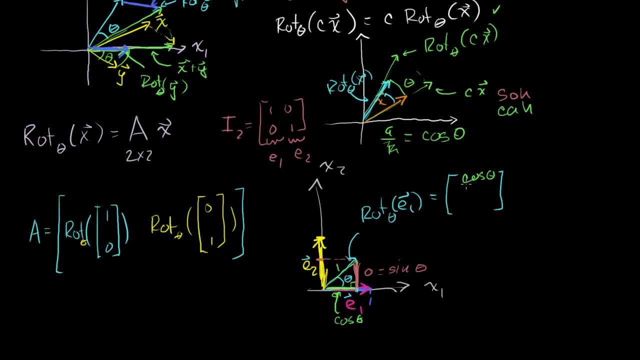 So the new rotated basis vector can be written as cosine of theta for its x component or for its horizontal component and sine of theta For its vertical component. This is the new rotated basis vector. Now, what about E2?? Well, we could do something very similar there. 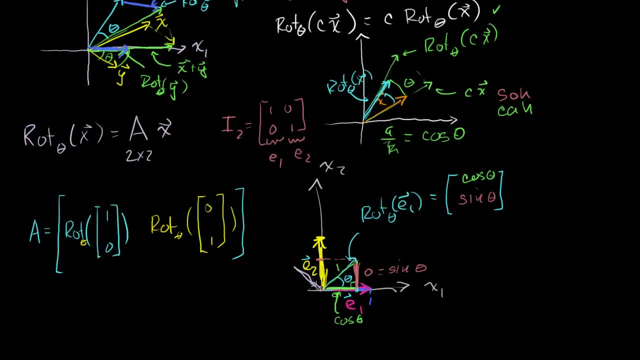 E2 is going to end up looking like this: when you rotate it by an angle of theta, It's going to look like that. That angle right there is theta. We can create a little right triangle right there. And so if we want to know its x coordinate, if we want to know 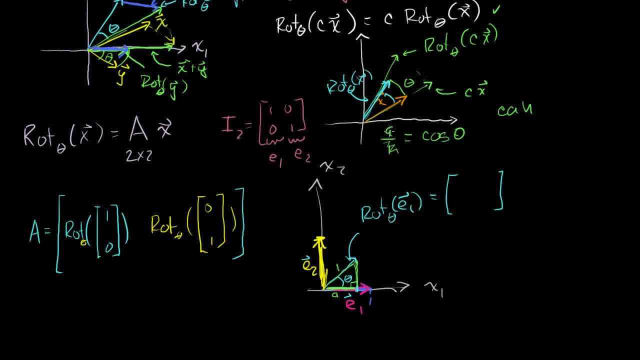 Well, we can obviously ignore that 1.. a divided by 1. is equal to cosine theta, which means that a is equal to cosine theta, which means that this length of our rotated vector is equal to cosine theta. Its horizontal component or its horizontal coordinate is: 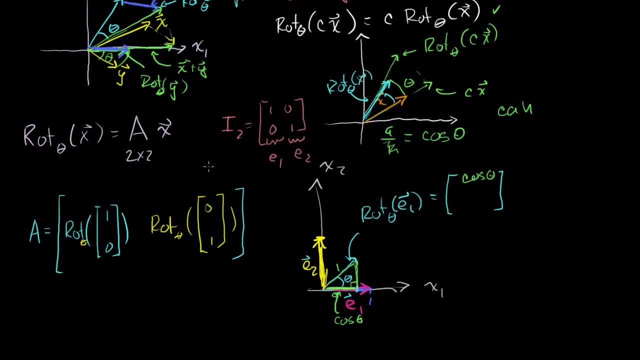 equal to cosine of theta. Now, if we take what's its vertical component going to be, it's going to be this height right here. It's going to be that height right there, which is the same thing as that height right there. 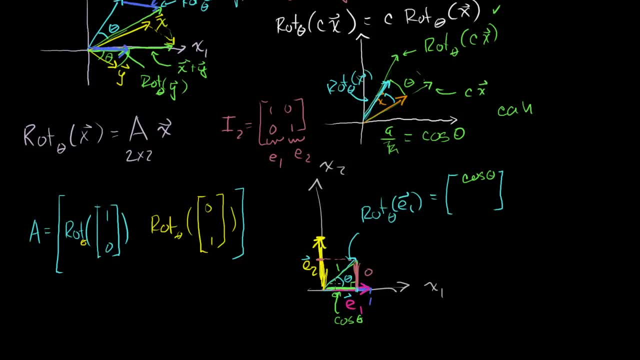 Or we could say sine of theta. Let me call this the opposite. Sine of theta is equal to the opposite over 1.. So this is going to be equal to sine of theta. This over 1, which is just this- is equal to sine of theta. 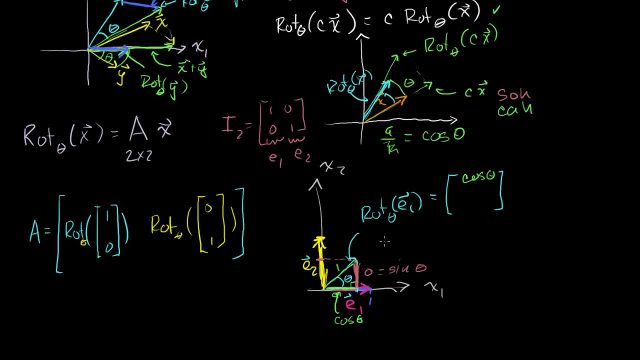 from SOH CAH TOA. So this vertical component is equal to sine of theta. So the new rotated basis vector can be written as cosine of theta for its x component or for its horizontal component and sine of theta for its horizontal component. 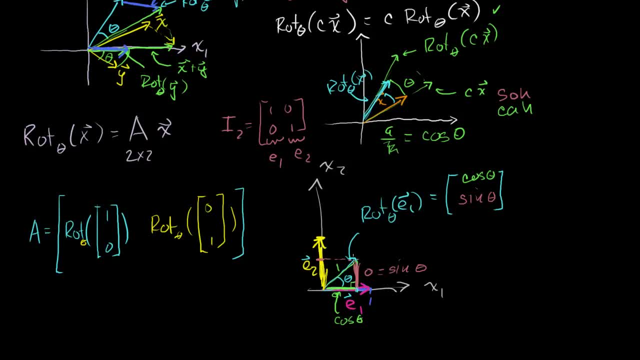 For its vertical component. This is the new rotated basis vector. Now what about E2?? Well, we could do something very similar there. E2's going to end up looking like this: when you rotate it by an angle of theta, It's going to look like that: 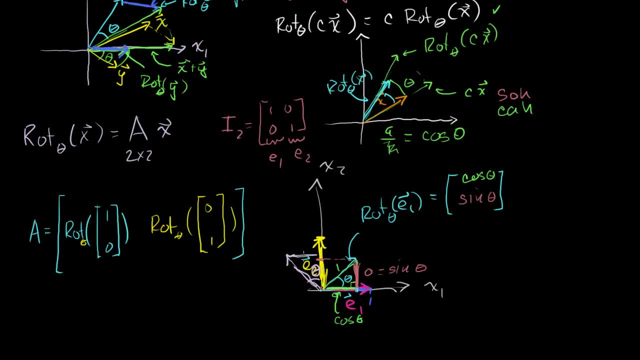 That angle, right there is theta. We can create a little right triangle right there, And so if we want to know its x-coordinate, so now we can take the x-coordinate If we want to know its x-coordinate, If we want to know its x-coordinate. 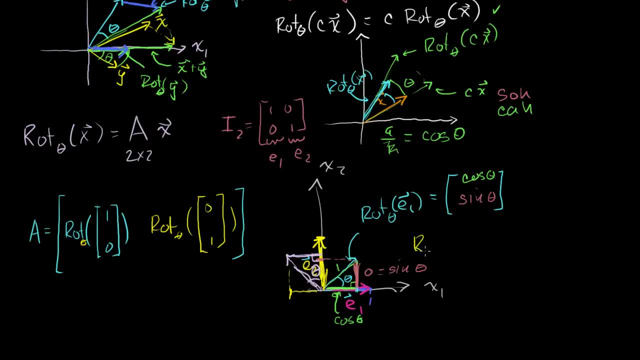 coordinate. so now we're concerned with the rotation through an angle of theta of e2, which is that right there of e2, this is e2, right there. This is going to be equal to what Its new x-coordinate or its first entry in this vector, if 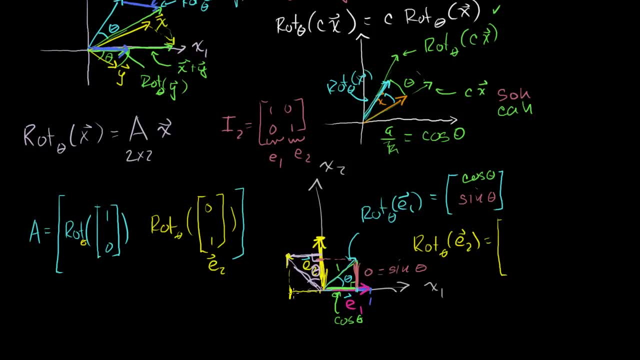 we wanted to draw it in standard position, or the point that it is specifying is going to be equal to this distance, which is equal to this distance on this triangle, but the coordinate's going to be the negative of this right. If this is a distance of 2, this coordinate is: 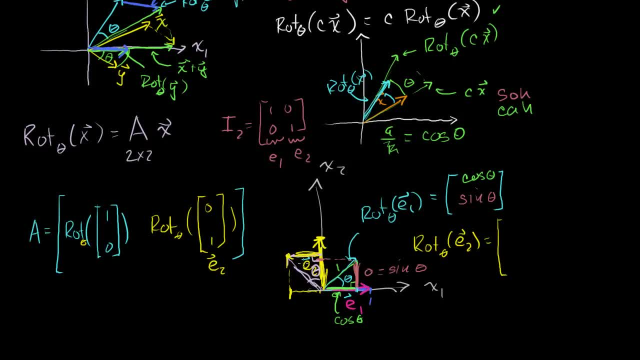 going to be minus 2.. So what's this? We have an angle. it's a right triangle. this is opposite to the angle. opposite over 1, opposite over our hypotenuse is equal to cosine of theta. So this opposite side is equal to the cosine of theta. 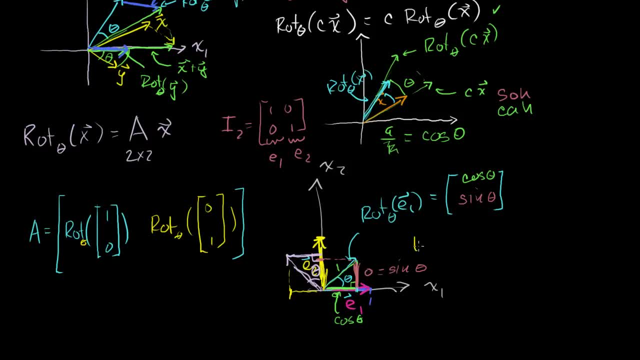 its x coordinate. so now we're concerned with the rotation through an angle of theta of E2, which is that right there of E2.. This is E2 right there. This is going to be equal to what Its new x coordinate or its first entry in this vector, if 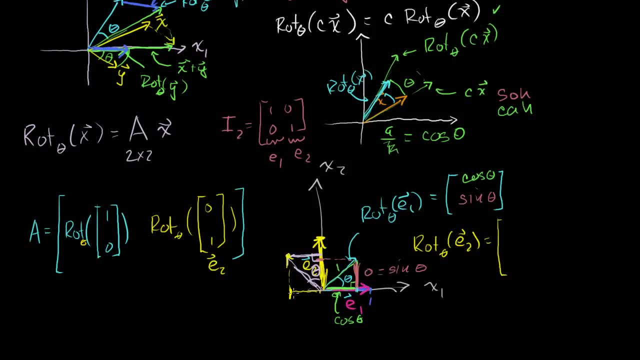 we wanted to draw it in standard position, or the point that it is specifying is going to be equal to this distance, which is equal to this distance on this triangle, but the coordinate's going to be the negative of this. If this is a distance of 2, this coordinate is going to be. 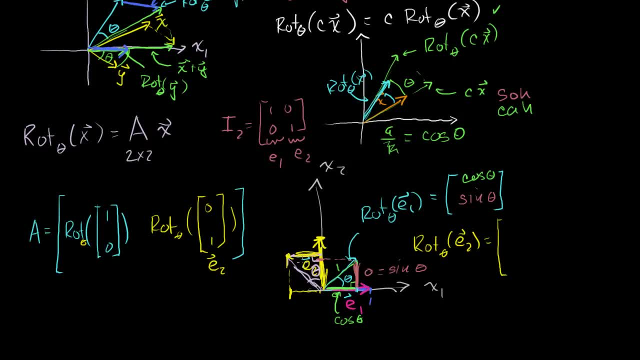 minus 2.. So what's this? We have an angle. It's a right triangle. This is opposite to the angle Opposite over 1, opposite over our hypotenuse is equal to cosine of theta. So this opposite side is equal to the cosine of theta. 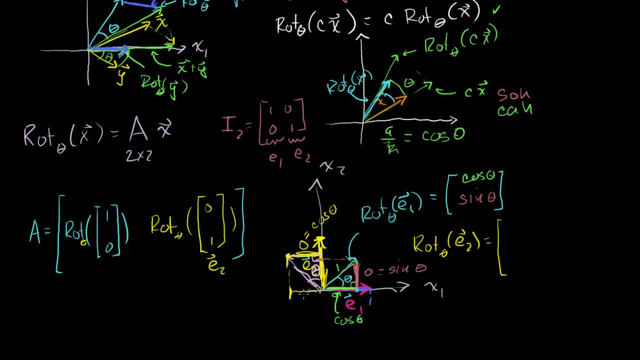 So the x coordinate right here. Oh sorry, My trigonometry is messing up. This is the opposite side. So katoa Sine is equal to opposite. Let me write it: Sine of theta is equal to opposite. 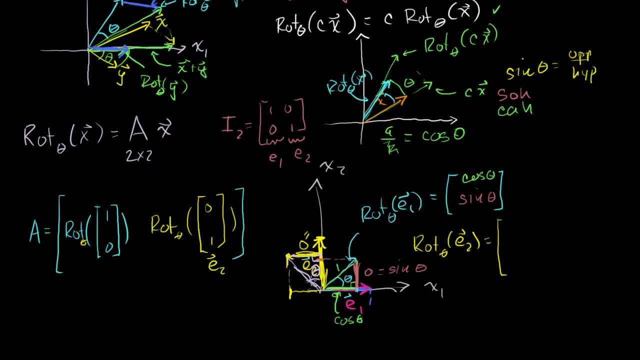 Opposite over hypotenuse. So the sine of theta, sine of this angle, is equal to this opposite over the hypotenuse. The hypotenuse is 1, has length 1, because these are the standard basis vectors. So this is equal to the sine of theta. 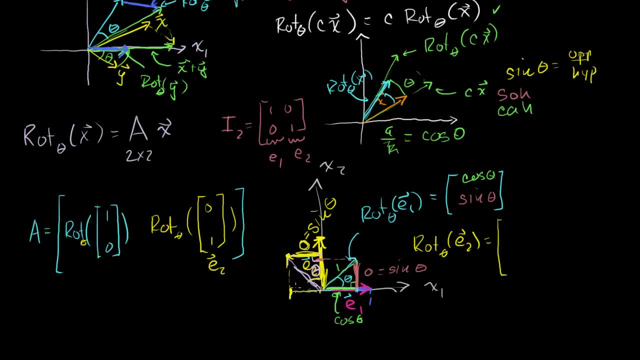 Now, this distance is equal to the sine of theta, but it's going in the negative direction, So it's going to be equal to the minus sine of theta. And then what's its new y component going to be of this rotated version of e2?? 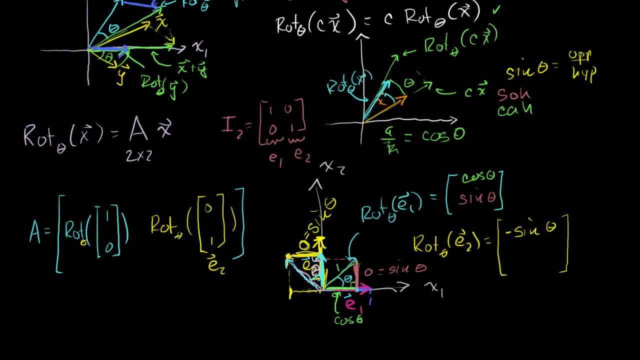 Well, we just look right here We have our angle. This is adjacent to the angle, This adjacent side over the hypotenuse, so adjacent over 1, which is just this adjacent right here, is just going to be equal to cosine of theta. 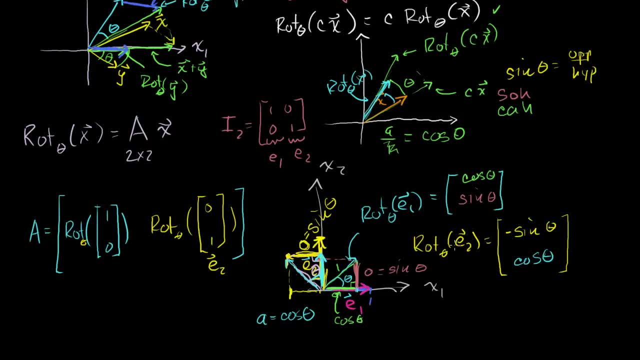 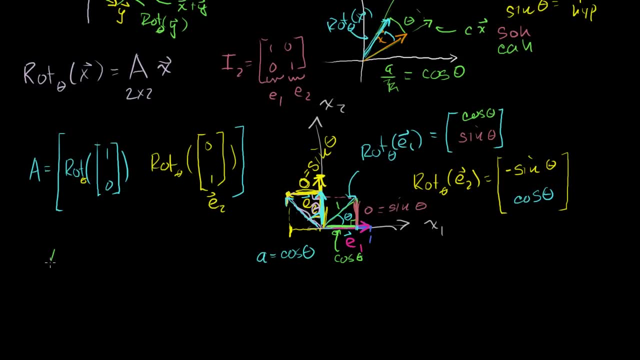 So its new y coordinate is going to be cosine of theta. So when we apply the transformation to each of our basis vectors, we get a is equal to the transformation applied to e1., Which is cosine of theta and sine of theta, And the transformation applied to e2,, which is minus sine of. 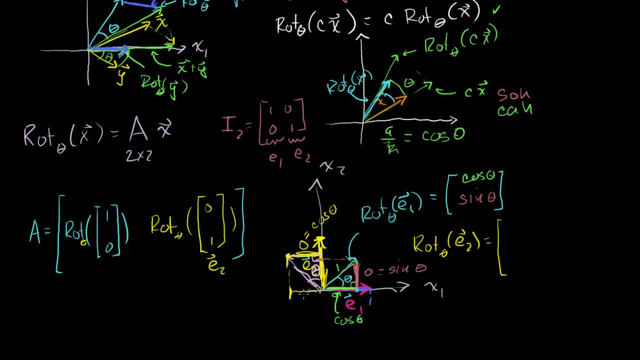 So the x-coordinate right here- oh sorry, my trigonometry is messing up- This is the opposite side. so katoa Sine is equal to opposite. let me write it because I was: sine of theta is equal to opposite. 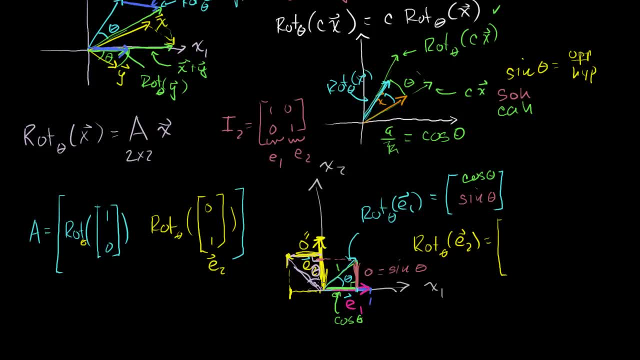 Over hypotenuse. So the sine of theta, sine of this angle, is equal to this opposite over the hypotenuse. The hypotenuse is 1,, has length 1,, because these are the standard basis vectors. So this is equal to the sine of theta. 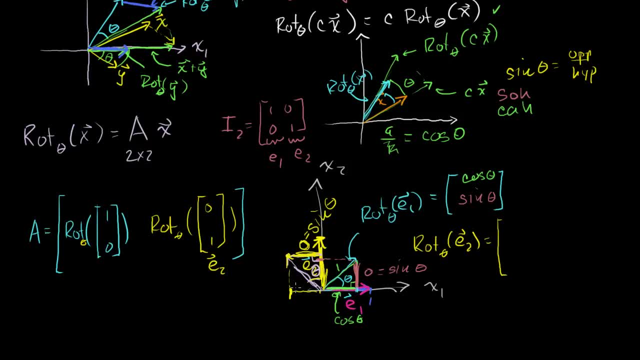 Now, this distance is equal to the sine of theta, but it's going in the negative direction, So it's going to be equal to the minus sine of theta. And then what's its new y-component going to be of this rotated version of e2?? 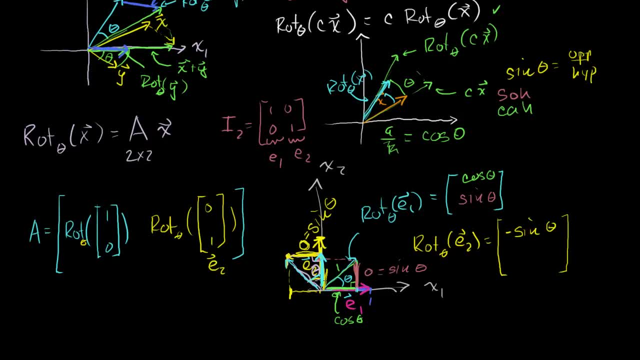 Well, we just look right here We have our angle. This is adjacent to the angle, This adjacent side over the hypotenuse, so adjacent over 1, which is just this adjacent right here, is just going to be equal to cosine of theta. 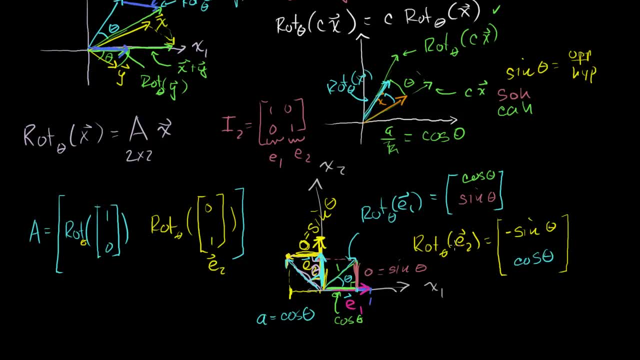 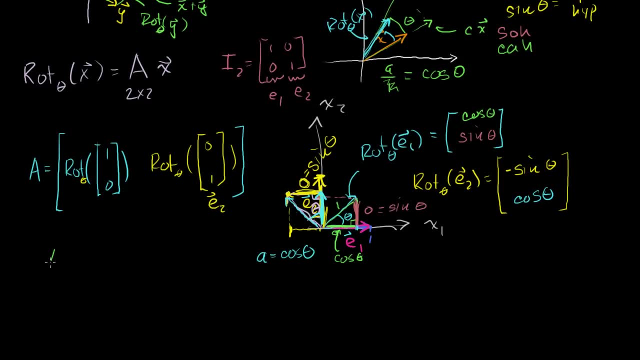 So its new y-coordinate is going to be cosine of theta. So when we apply the transformation to each of our basis vectors, we get a is equal to the transformation applied to e1.. Which is Which is cosine of theta and sine of theta. 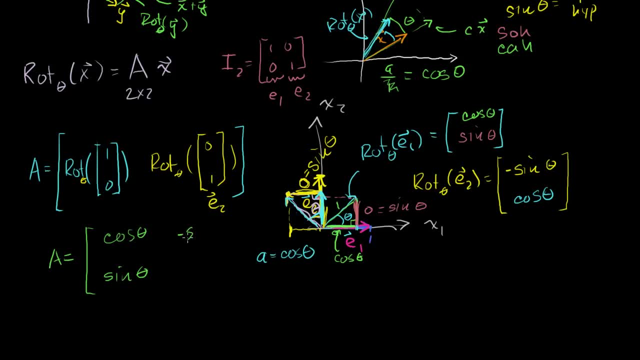 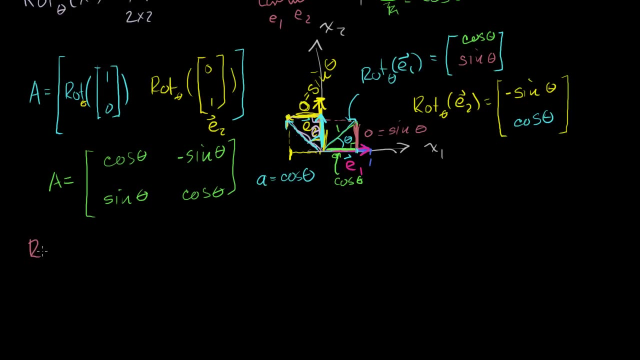 And the transformation applied to e2, which is minus sine of theta, times the cosine of theta. So now this is a big result. We've now been able to mathematically specify our rotation transformation using a matrix. So we can now say that the rotation transformation and 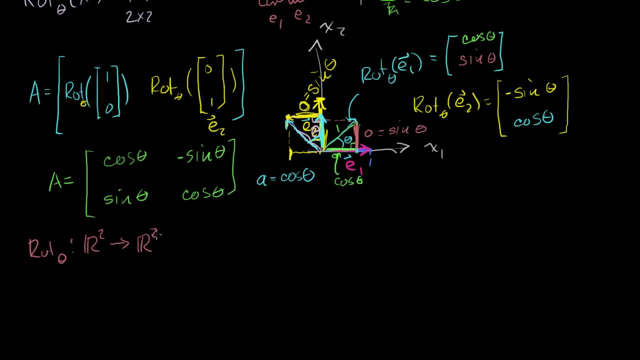 it's a transformation from R2 to R2, it's a function. We can say that the rotation through an angle of theta of any vector x in our domain is equal to the matrix cosine of theta. sine of theta minus sine of theta. cosine of theta. 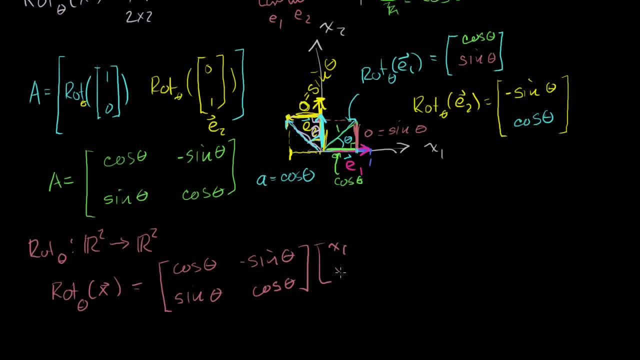 times your vector in your domain, times x1 and x2.. And you might be saying, oh, Sal, you know we did all this work and that's kind of neat, but how do I apply this? You know, I still have all these cosines of thetas and 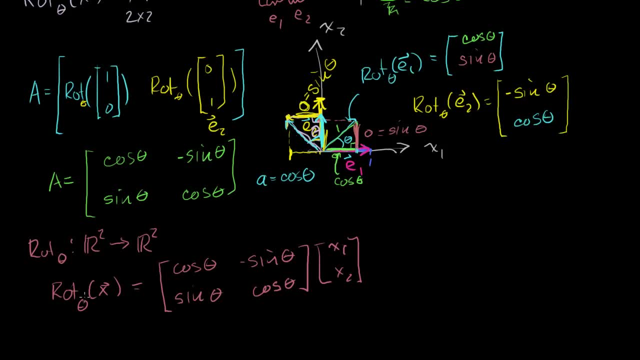 sines of thetas there. How do I do it? Well, what you do is you pick an angle you want to rotate to and just evaluate these, and you'll just have a normal matrix with numbers in it. So let's say that we wanted to rotate through an angle of 45. 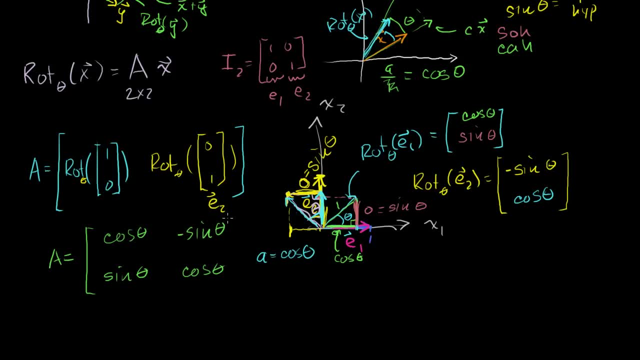 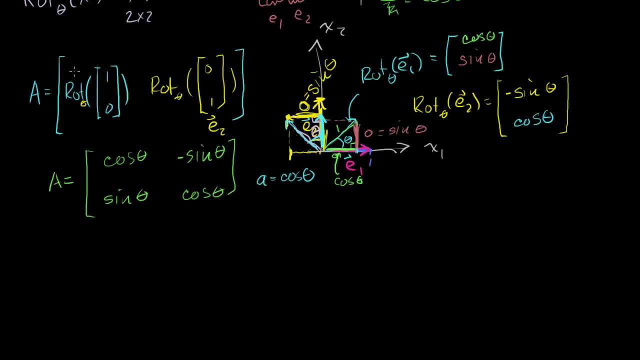 theta times the cosine of theta. So now this is a big result. We've now been able to mathematically specify our rotation transformation using a matrix. So we can now say that the rotation transformation- and it's a transformation from R2 to R2, it's a function. 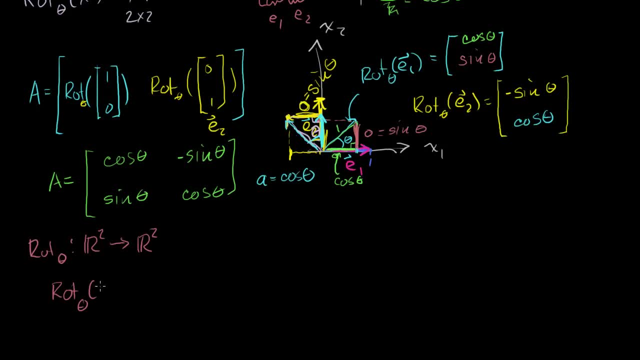 We can say that the rotation through an angle of theta of any vector x in our domain is equal to the matrix cosine of theta, sine of theta, minus, sine of theta, cosine of theta times your vector in your domain, times x1 and x2.. 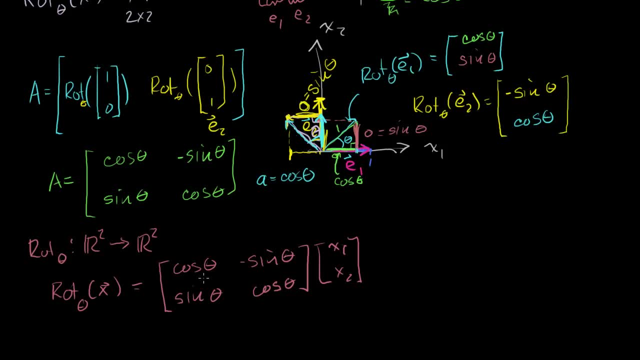 And you might be saying, oh, Sal, you know we did all this work and that's kind of neat, but how do I apply this? You know, I still have all these cosines of thetas and sines of thetas there. 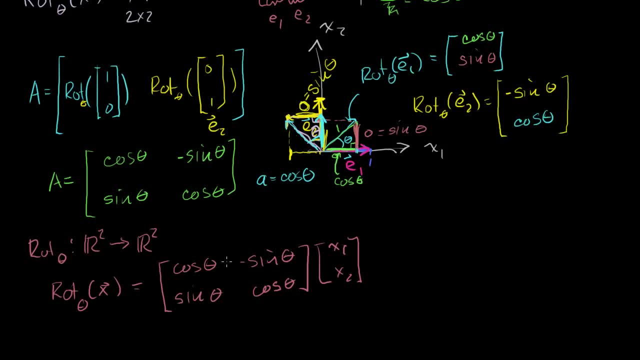 How do I do it? Well, what you do is you pick an angle you want to rotate to and just evaluate these, and you'll just have a normal matrix with numbers in it. So let's say that we wanted to rotate through an angle of 45. 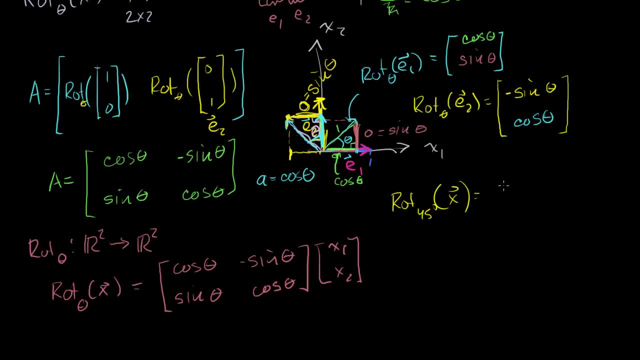 degrees, some vector. Well, this is going to be equal to what We just apply, or we evaluate each of these ratios at 45 degrees. The cosine of 45 degrees is square root of 2 over 2.. Sine of 45 degrees is square root of 2 over 2.. 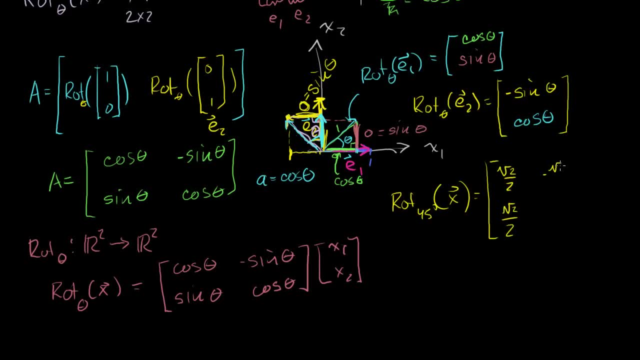 Sine of 45 is square root of 2.. We have a minus there, so minus square root of 2 over 2.. And then cosine is just another square root of 2 over 2.. So then we multiply: it times our vector x. 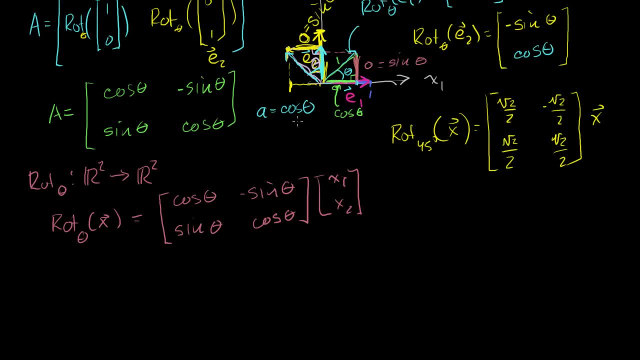 So this matrix, if we multiply it, times any vector x literally. so if we have some coordinates right here, and let's say that I were to I don't know, let's say I were to have a bunch of vectors, Let's specify some square here. 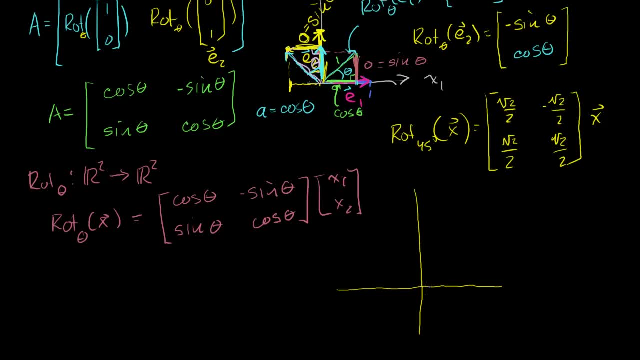 Let me see if I can do it properly. Well, maybe it has some triangle here. Maybe that'll be a little easier for me to draw. I'll do a square. Let's say it has some square here. Let's say I have some square here in my domain. 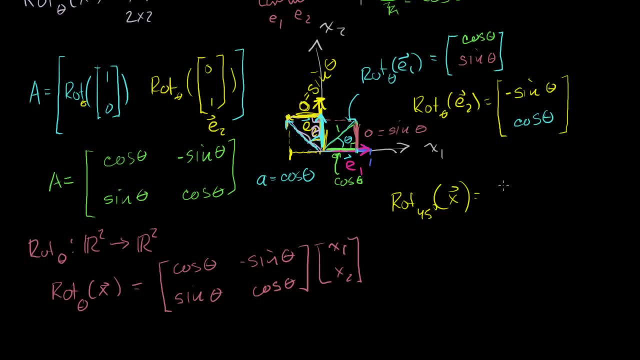 degrees, some vector. Well, this is going to be equal to what We just apply, or we evaluate each of these ratios at 45 degrees. The cosine of 45 degrees is square root of 2 over 2.. Sine of 45 degrees is square root of 2 over 2.. 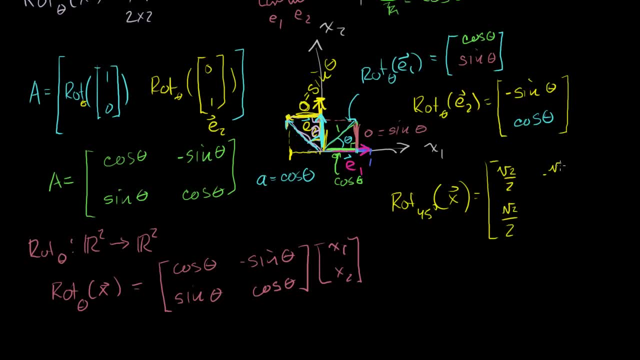 Sine of 45 is square root of 2 over 2.. We have a minus there, so minus square root of 2 over 2.. And then cosine is just another square root of 2 over 2.. So then we multiply: it times our vector x. 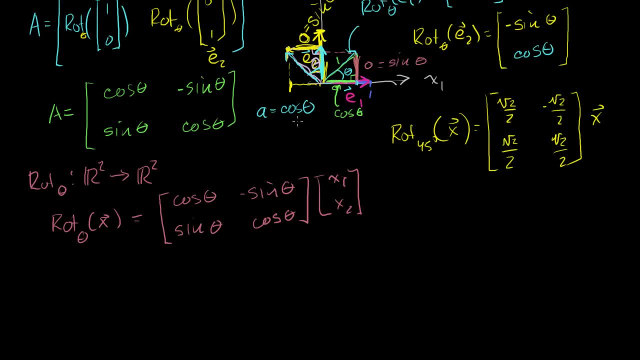 So this matrix, if we multiply it, times any vector x literally. so if we have some coordinates right here, and let's say that I were to I don't know, let's say I were to have a bunch of vectors, Let's specify some square here. 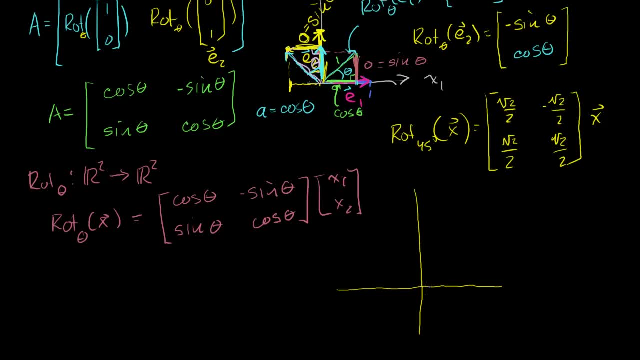 Let me see if I can do it properly. Well, maybe it has some triangle here. Maybe that'll be a little easier for me to draw. I'll do a square. Let's say it has some square here. Let's say I have some square here in my domain. 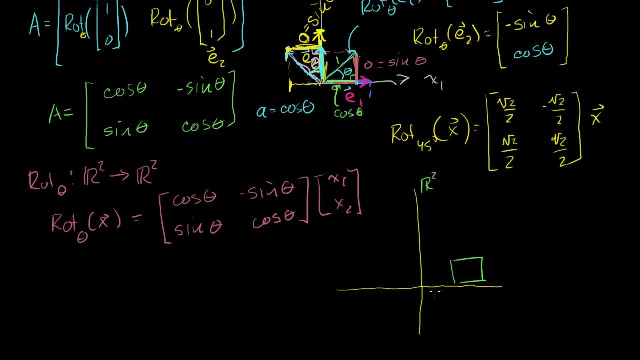 So this is an r2.. Now, when I apply, if I literally multiply this times each of the basis vectors, or actually all of the vectors that specify this set, here, I will get, When I transform it, I'll get- a rotated version of this by 45. 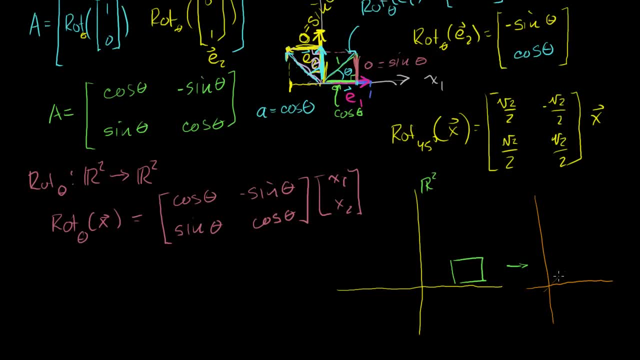 degrees, Just to draw it. I'll actually draw a little 45 degree angle right there And then it will map it to this image right there, Which is a pretty neat result If you ever attempted to write any computer game that involves. 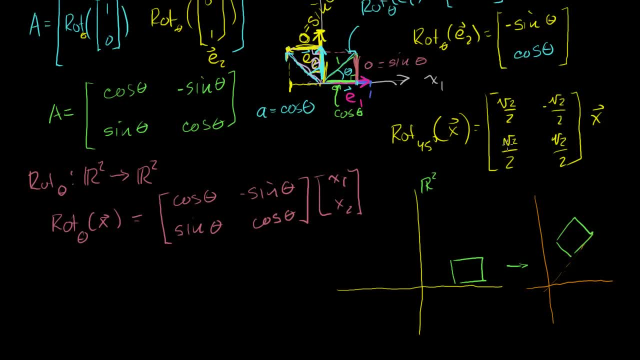 marbles or pinballs going around. this is a very useful thing to know. How do you rotate things? In the future we'll talk about other types of transformations, But this is a super useful one. and this is super hard to do, and I remember the first time I wrote a computer. 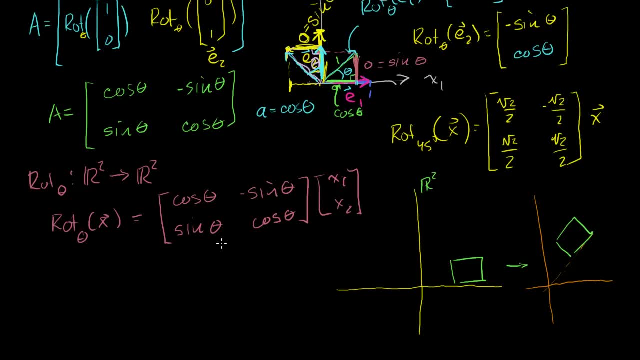 program that tried to do this type of thing. I just did it by hand. But when you have this tool at your disposal, all you have to do is evaluate this matrix at the angle you want to rotate by, and then multiply it times your position vectors. 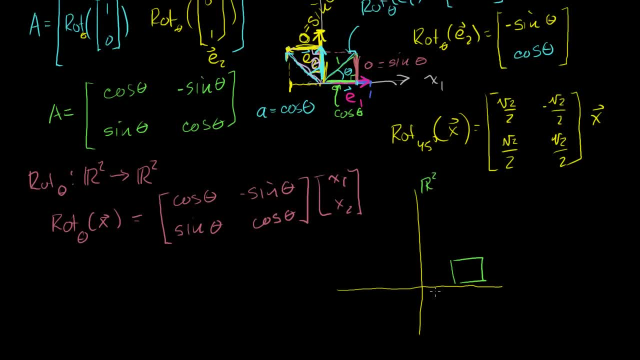 So this is an r2.. Now, when I apply, if I literally multiply this times each of the basis vectors, or actually all of the vectors that specify this set, here, I will get, When I transform it, I'll get- a rotated version of this by 45. 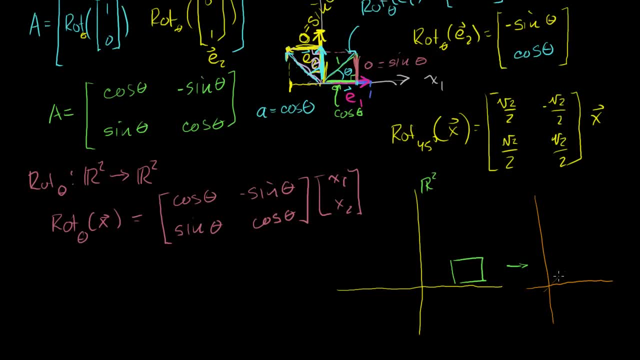 degrees Just to draw it. I'll actually draw a little 45 degree angle right there And then it will map it to this image right there, Which is a pretty neat result. And if you ever attempted to write any computer game that involves marbles or pin balls going around, this is a very 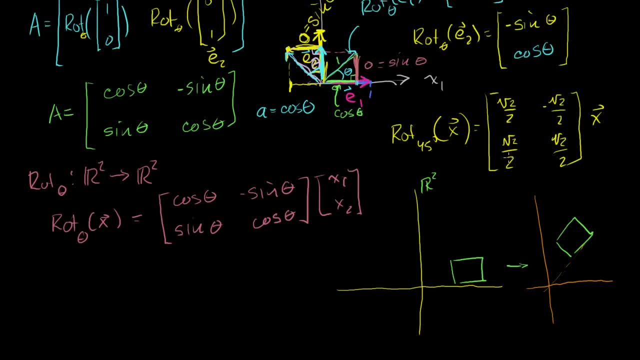 useful thing to know of how do you rotate things, and in the future we'll talk about other types of transformations, But This is a super useful one. This is super hard to do And I remember the first time I wrote a computer program that 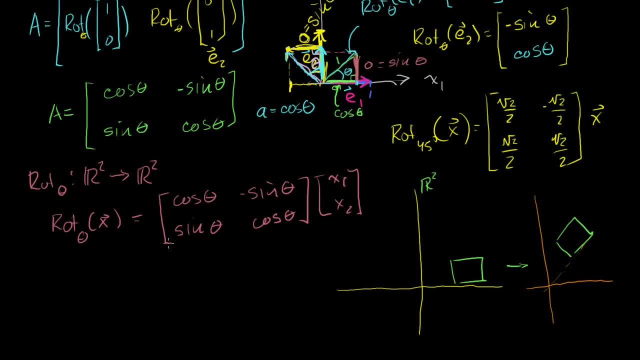 tried to do this type of thing. I just did it by hand. But when you have this tool at your disposal, all you have to do is evaluate this matrix at the angle you want to rotate by, and then multiply it times your position. vectors. 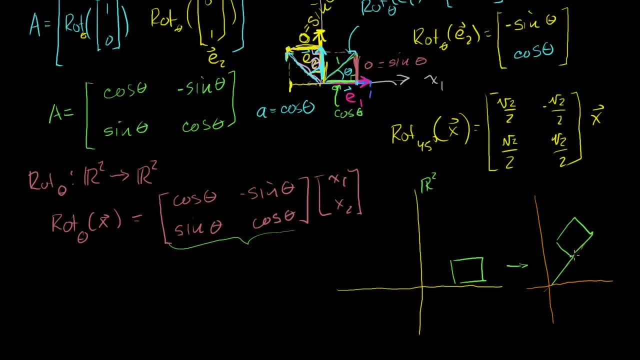 And so obviously you have a bunch of position vectors here, but here you can just do it times the vertices and then you can say OK, and everything else is just connect the dots between them And then you have your rotated image. And just to be clear, these are the points specified by a. 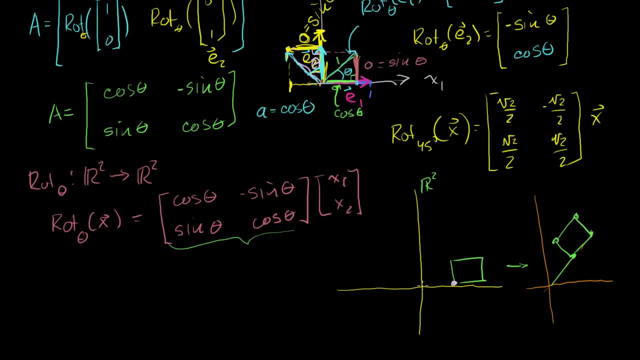 set of vectors- And I always want to make this clear- right, This point right here is specified by some position vector that looks like that: When you apply the rotation on 45 degrees of that vector, this vector then looks like this: And the vector that specified this corner right here, let me 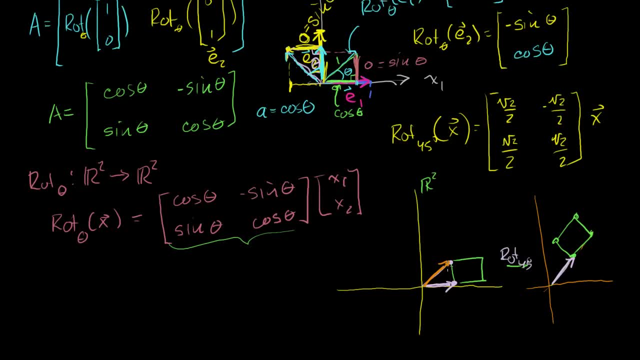 do it in a different color that specified this corner right here. when you rotate it by 45 degrees, then becomes this vector And the vector that specified that corner over there that now becomes this vector. That's what's actually being mapped, or? 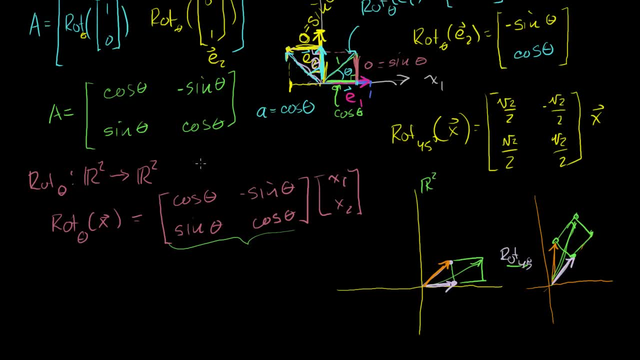 actually being transformed. Anyway, hopefully you found this pretty neat. I thought this was a- at least for me, this was kind of the first really neat transformation. You can already start thinking about how to extend this into multiple dimensions, especially three-dimensionals. 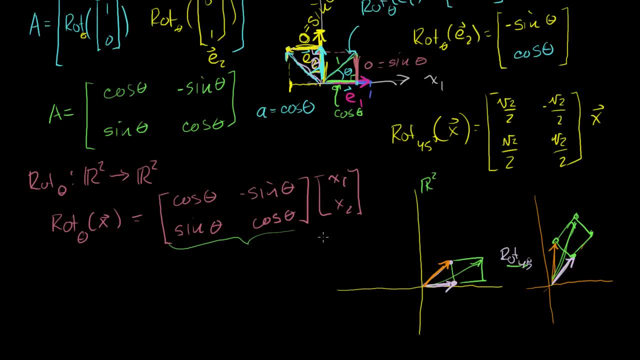 If you ever try to actually do it by hand, three-dimensional rotation becomes very confusing. But in the next video we'll actually figure out a way to do three-dimensional rotations around certain axes. See you then, Bye, Bye, Bye, Bye.